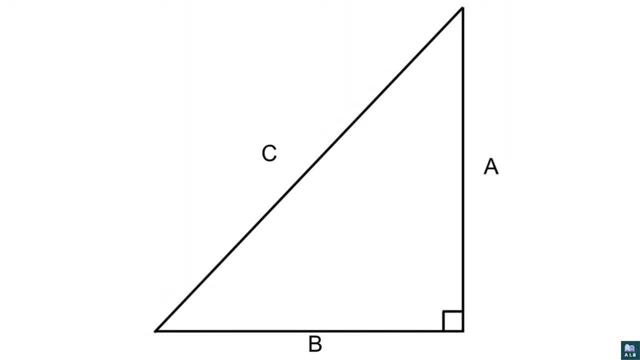 of a right triangle. So if you calculate something and it works out to be smaller than a or b, you've done something wrong. And we also know that, because it is opposite the 90 degree angle, so it will always be the longest side. 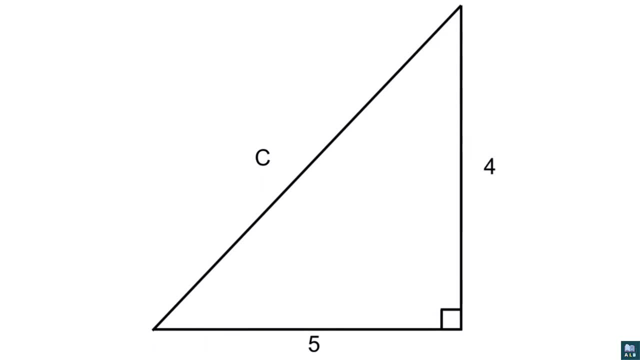 So let's throw something in here. I'm just going to say I'm going to do it. So what you values at this, a and b have given the values of 4 and 5.. We're trying to determine what c is here Now using Pythagoras' theorem. we know that a squared plus b squared is equal. 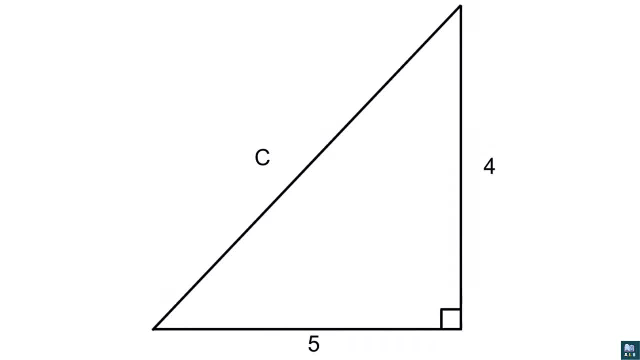 to c squared. so we know that the formula is going to be: 4 squared plus 5 squared is equal to c squared. So, now that we've determined that c squared is equal to 4 squared plus 5 squared, let's get rid of these 4 squareds and 5 squareds. We know that 4 squared, which 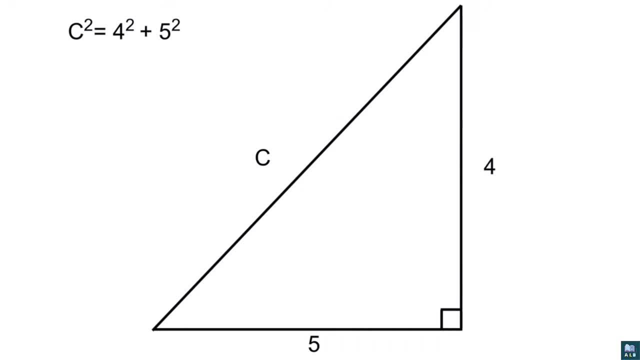 is 4 times 4, is equal to 16 plus 5 times 5,, which is equal to 25.. c squared is equal to 16 plus 25.. Now that I've determined c squared is equal to 16 plus 25,, why don't? 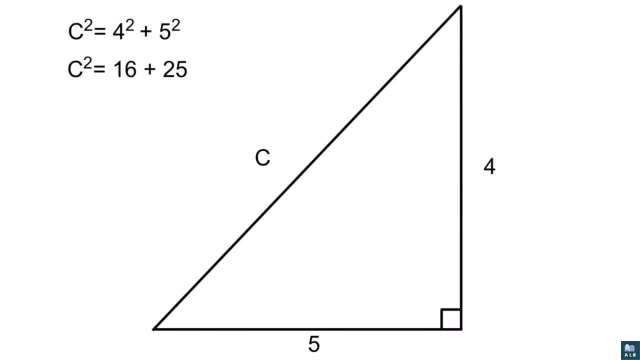 we add 16 and 25 together and be done with it. So c squared is equal to 41.. Now that I've determined that c squared is equal to 41, I'm not looking for c squared, I am looking for c. So we need to get rid of our square system. 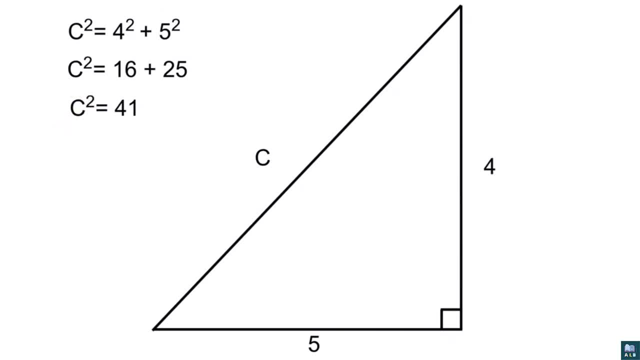 somehow, and like I said before, we have to square root this side to get rid of the square. whatever we do to this side, we have to do to this side. so C is equal to the square root of 41. so go ahead and punch it in your calculator: C is equal. 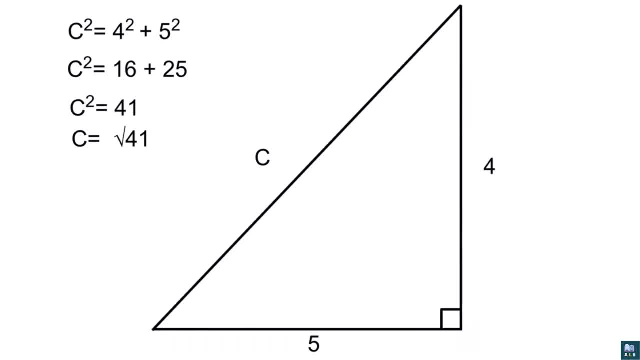 to the square root of 41 and you're gonna work out that C is equal to six point four. so congratulations, you've just solved for the hypotenuse, which is this C, and so let's get rid of C and throw the answer in there. so there we go. now we've determined that four squared plus five squared is equal. 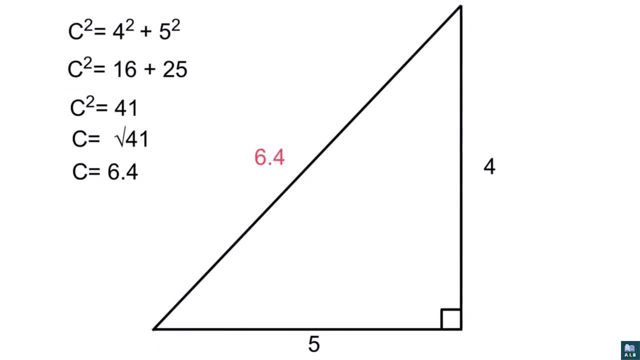 to six point four squared. now what do we do, though, if we have a hypotenuse side in one of these sides and need to determine this side, as we did before? let's throw some numbers at it. I've got. the hypotenuse is four hundred and fifty. 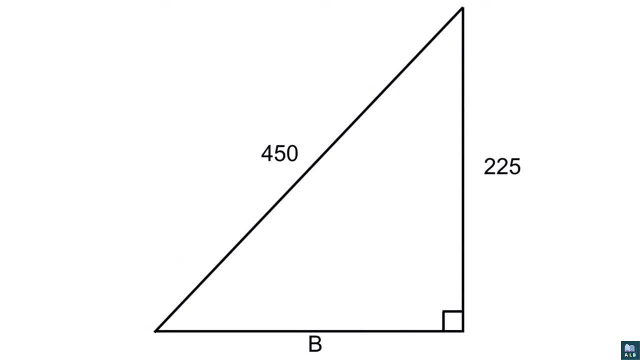 and the B side or the half side. I'm going to draw the half side. I'm going to draw the half side and the the A side is 225,. sorry, the A side, And now we want to determine what the B is, So what we're. 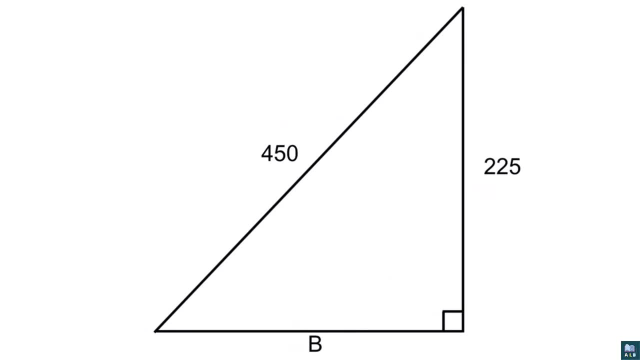 going to do is: let's plug into the formula what we know. We know that the formula is: A squared plus B squared equals C squared, or C squared is equal to A squared plus B squared. So let's throw that in there. We know that 450 squared is equal to 225 squared plus B squared. Let's throw that into. 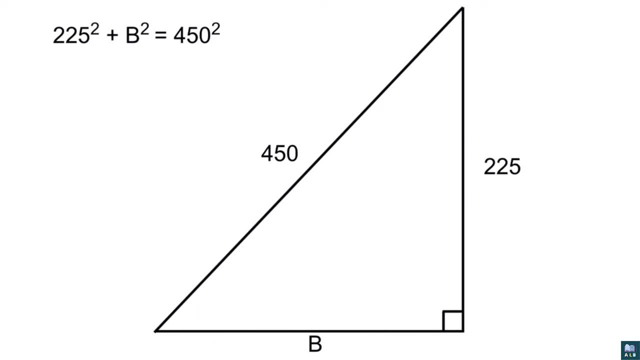 our formula. Okay. so we've got that. 225 squared plus B squared is equal to 450 squared. Now we need to get B alone. So what we have to do is we have to subtract this 225 squared out of there. 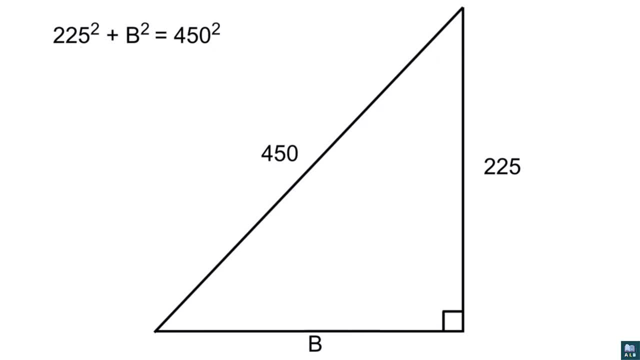 Now, even before we do that, let's get rid of these squares. Let's figure out what 225 squared is and what 450 squared is and deal with those numbers first. So we see that 225 squared actually works out to be 50,625.. That's a big number. Plus B squared is equal to 202,500.. Now we need to get 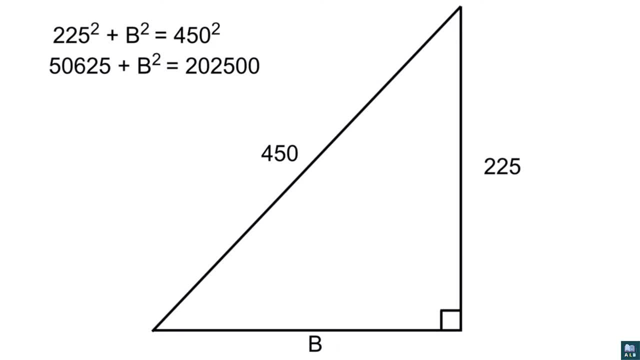 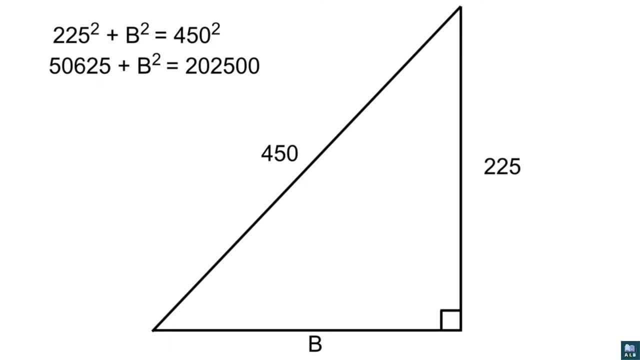 that we have to subtract this to get rid of it. as with any equation, whatever you do to one side of the equation, you have to do the other. so b squared is going to equal 202 500 minus 50 625. so all we've done is we've moved the equation around here so we have: b squared is equal to. 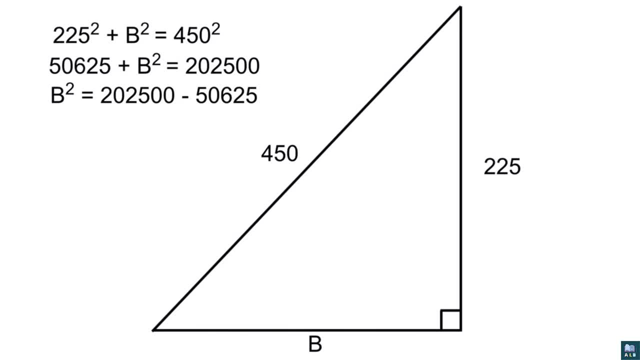 202 500 minus 50 625, which works out to be 151 875. so we're getting closer to our answer. b squared is equal to 151 875, as before. we need to get rid of the square. that doesn't do us any good. let's square aquilo. yes, squared. 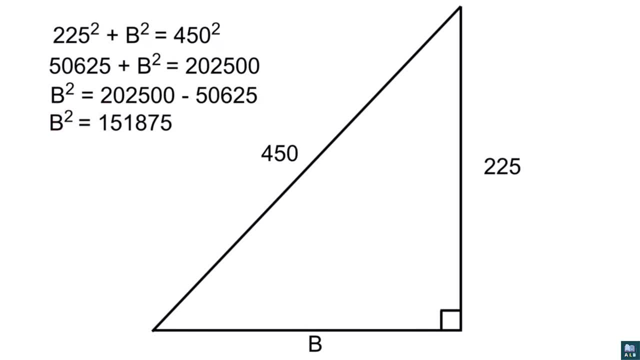 root the b squared and then let's square root 151,875 and get our answer, because it's going to be: b is equal to the square root of 151,875.. So we're starting to see the answer get closer and closer here. b is equal to the square root of. 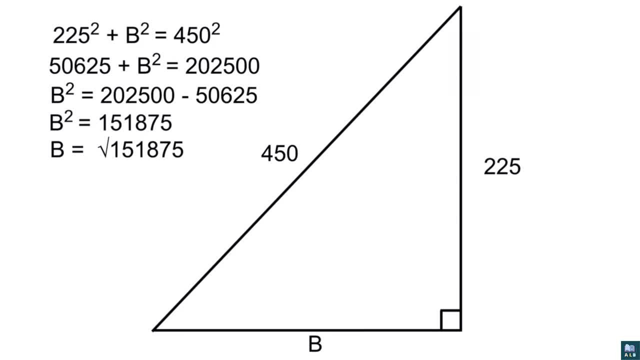 151,875. punch that into your calculator and we get our answer of 389.7.. So we have determined that 450 squared minus 225 squared gives us 389.7 squared. That is determined the size of b, And that basically completes our walkthrough of. 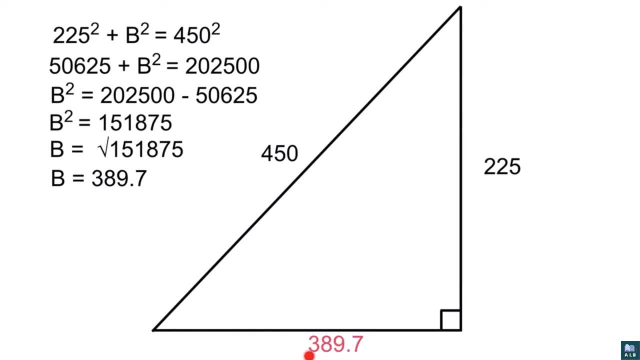 Pythagoras' theorem. It doesn't matter if you have this side and this side, you can go: a squared plus b squared is equal to c squared, or if you have this side, you're just going: c squared minus this side is equal to this squared, or c squared minus this squared is equal. 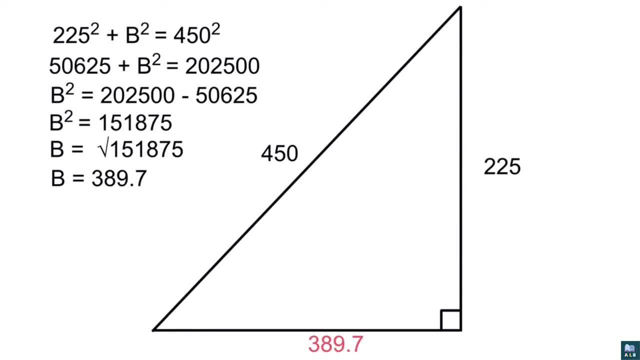 to this squared. It's not too shabby at all. It's not too hard to walk through. This should just be a review from grade 12, or not even grade 12, probably grade 10 geometry. In our next video we're going to start getting into some more trig. 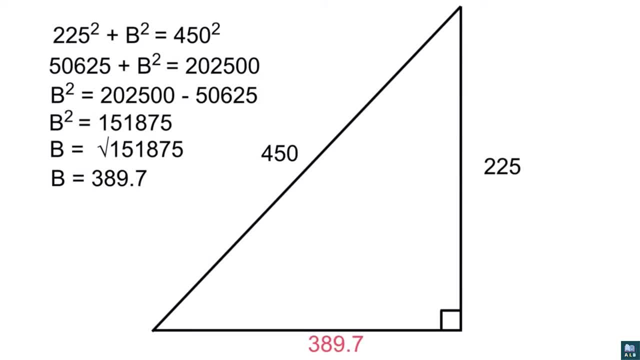 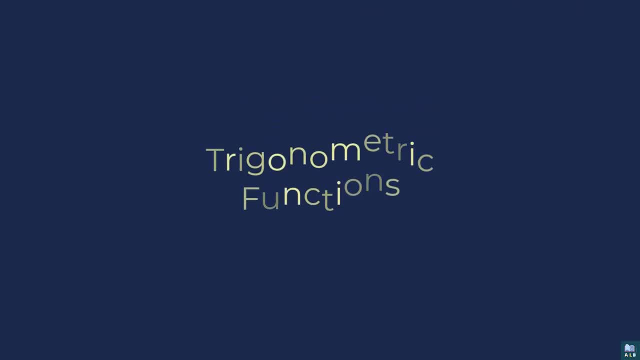 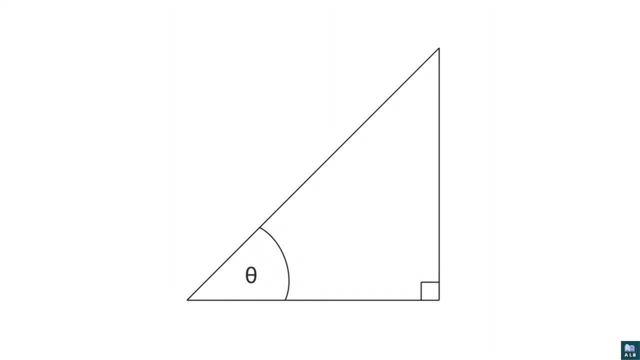 functions, talking about the ratios of sides and starting getting into sine cosine and tangent. In this video we'll start getting into trig functions, sine cosine and tangent. But before we do that, what we have to do is name the sides of the triangle. We have this side. 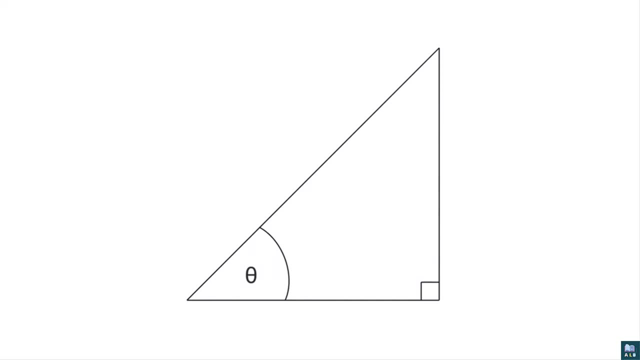 here, which we discussed in the last one, is always going to be called the hypotenuse, But this fellow and this fellow, they have different names. Now it's all going to be based off what we call our designate angle. Now you see this little funky Greek symbol. 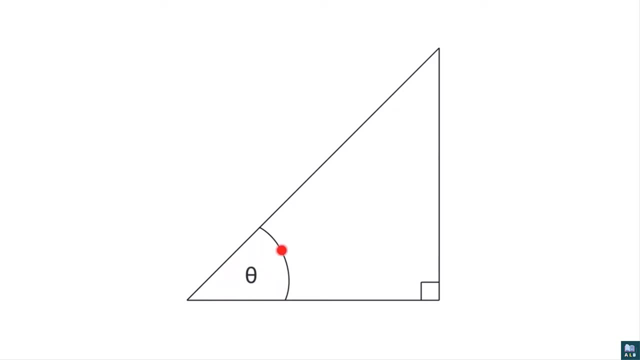 here we call that theta and in this case this is my designate angle. So let's walk through how I name these sides based off the fact that this here is my designate angle. We know that this is the hypotenuse. There we go. Now we have. 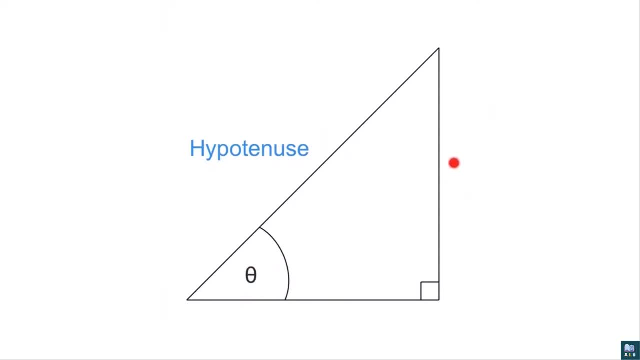 our designate angle sitting here and we have our side over here which is sitting opposite of that. Guess what that side is called. Yep, that's right, that's our opposite side. Now we also have this side that's sitting down here, that is sitting adjacent to the. 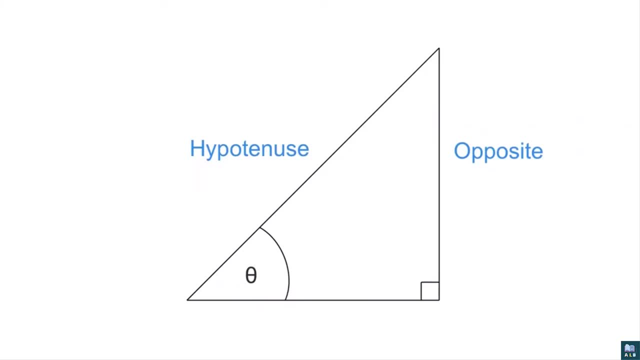 theta symbol or the designate angle, and you'll notice I said adjacent, So guess what that name is going to be. Yep, you guessed it adjacent. Now that's all based on the fact that this theta or this designate angle is sitting here. Now what if we moved it up to this side here? 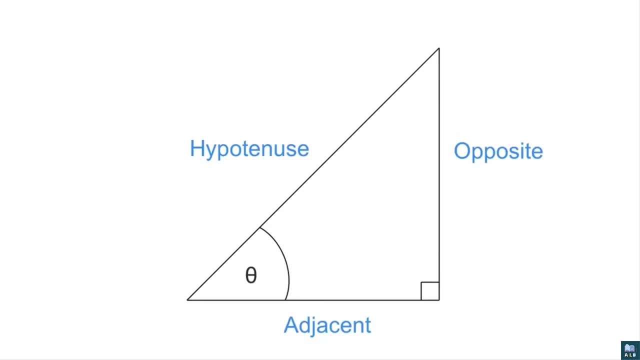 would that change things 100%? yes, Now the hypotenuse is always going to be the hypotenuse because it's the longest side, so that didn't change. but this side and this side are going to change names. Let's move that theta up to here, Our designate. 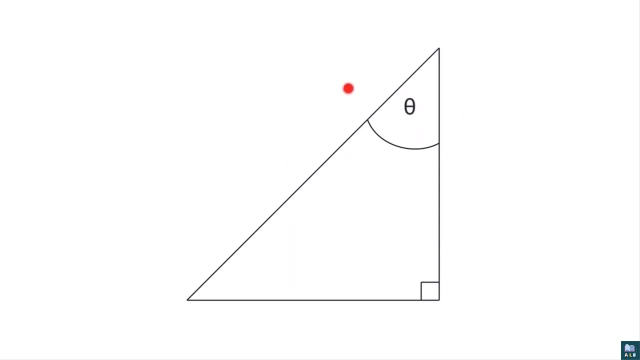 angle is now up, top, up top, which means that this stays the hypotenuse. Now, here comes the changes. Now, this side, which used to be the adjacent, is now the side that is opposite our theta, or our designate angle, and this side over here, which once sat. 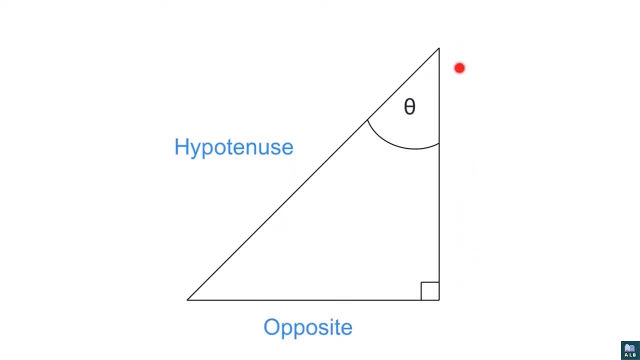 opposite. our designate angle is now sitting adjacent to our designate angle. Now, when we start dealing with these things, we're going to talk about the ratios of the sides of the triangle and how they're related to our designate angle. They all have ratios, Each side here. 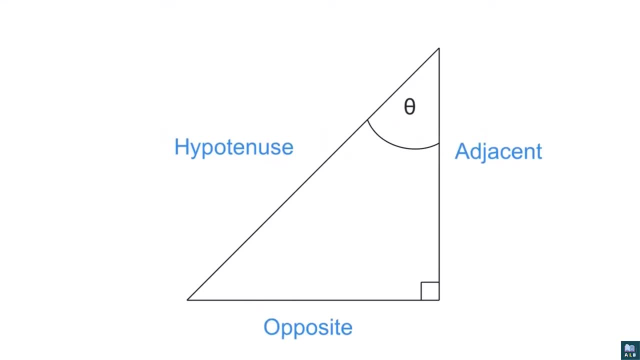 has a ratio which will help us determine what this angle is. So let's flip this triangle back on to its side here and make this our designated angle and talk about these ratios. Now, on this side, I've got my designated angle. This will be my opposite, This is my hypotenuse and this is my 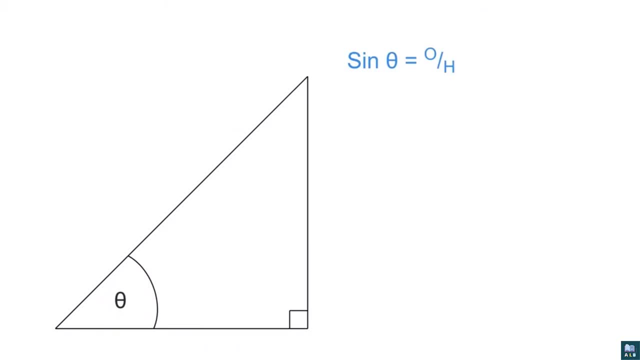 adjacent. If I want to figure out what this angle is, somebody who's smarter than all of us has determined that the sine of this angle is equal to the ratio of my opposite side over my hypotenuse. Now, that's not where it ends. There's others. We also could say that the cos of this angle, or the 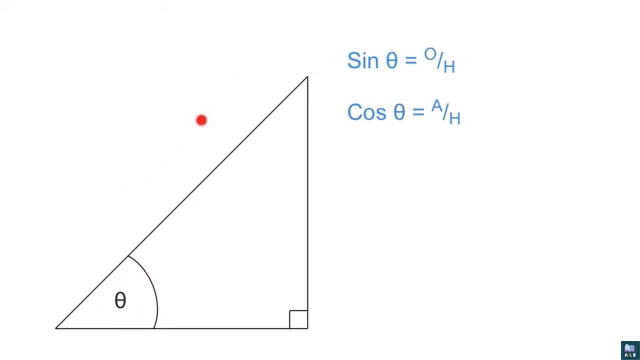 cosine of this angle is equal to our adjacent over our hypotenuse. Say that five times real fast. The ratio of this side over this side. That is our cosine. We've got one more. We can say that the tangent of our designated angle, or the tangent of theta, is equal to our opposite over our. 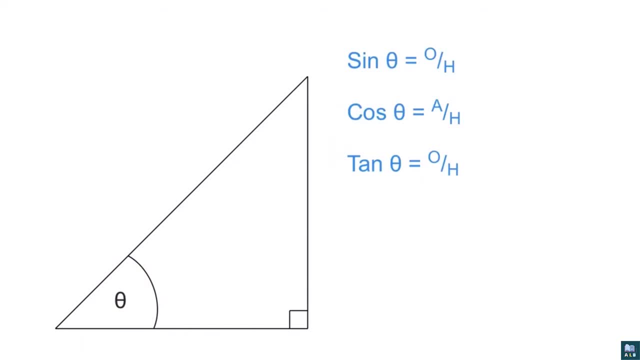 hypotenuse. Now that's not where it ends. There's others. We also could say that the cosine of this angle or the tangent of theta is equal to our adjacent over our hypotenuse. Those are the three trig functions we're going to use. We're going to use sine, cosine and tangent. There's an easy. 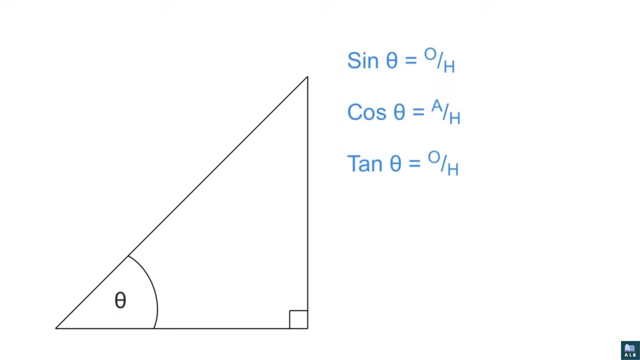 way to remember the ratios. Instead of having to have this hard memorization problem, we can just come up with this mnemonic, and it is this. I'm sure a lot of you guys know it: SOH, CAH, TOA, SOH. 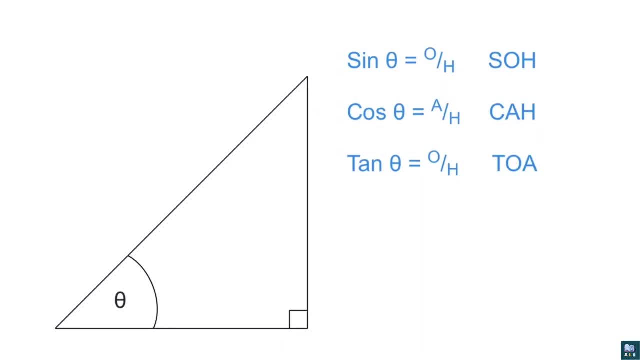 sine is opposite over hypotenuse. CAH cosine is adjacent over hypotenuse. TOA tangent is opposite over adjacent. Now, you should never forget that. I'm sure you actually already knew that. coming into this Now, as we did in the previous video, let's start throwing some numbers at this and playing. 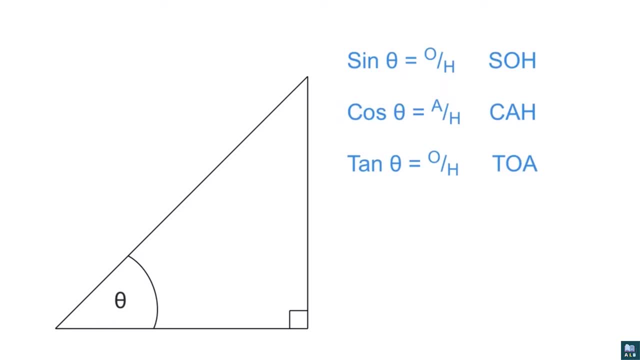 with this and figuring out how we can determine angles. So let's use the common three, four, five triangle. here You can use Pythagoras' theorem to determine that three squared plus four squared equals five squared. It all plays out from the last video. You can prove that. Now what we're. 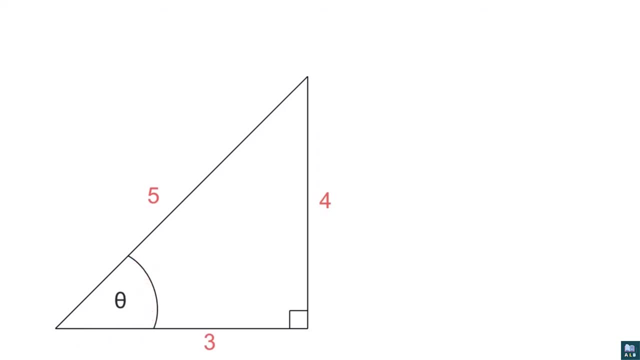 trying to do is determine what this angle is, because that becomes very important to us in electrical theory later on. Now we can use any of those three trig functions- sine, cosine or tangent. So what we're going to do is walk through with all three. Let's start out with sine. The sine of this angle is: 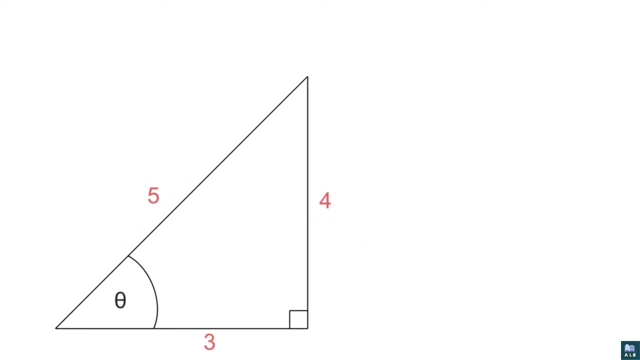 equal to our opposite over our hypotenuse. So sine theta is equal to four over five. So let's just write that off on the side. there The sine of theta is equal to four over five. Now, let's get rid of this. The sine of theta is equal to four divided by five, which is 0.8.. So now comes the tricky part. 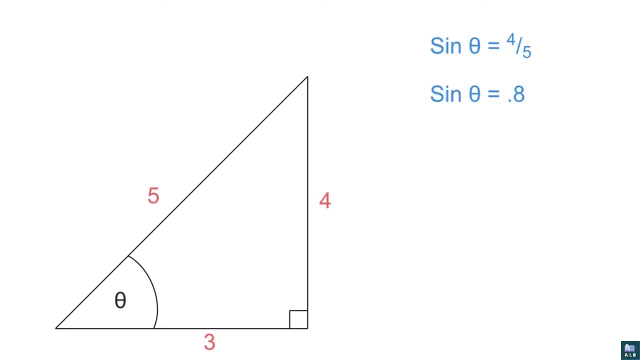 We've got sine of theta is equal to 0.8, but we don't want that sign there. We want to get rid of that. We want just to figure out what the theta is or what the angle is, So what we're going to have. 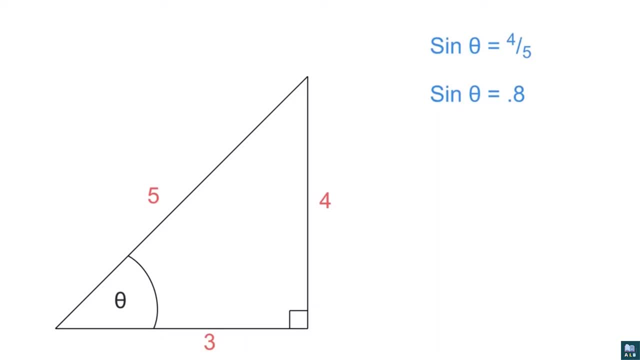 to do is use our calculators, And if you take a look at your calculator, you should have trigonometry functions on your calculator. If you don't, then you've got the wrong calculator on you. If you have a smartphone, you could probably just take your calculator out, and if you lay 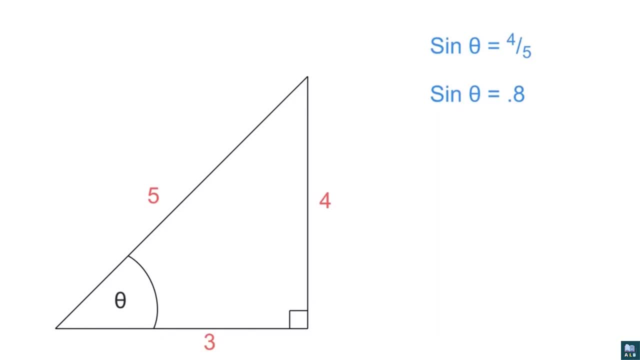 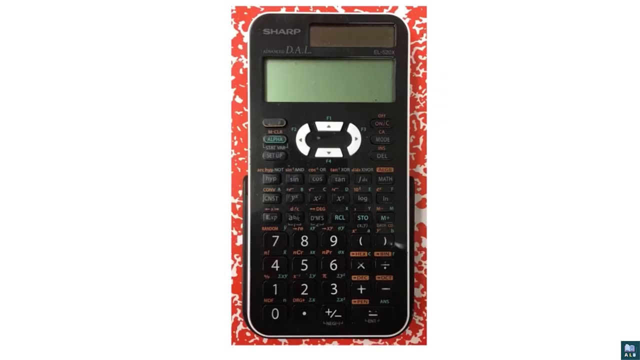 it on its side. it should pull up some trig functions. But let me show you a picture of the calculator that I use when I'm teaching this stuff. What we need to do is find your inverse sine. Now, if you look at this calculator here, I've got my trig functions up here. Sine cosine. 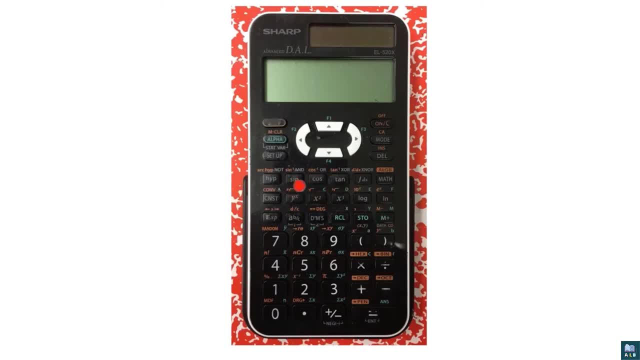 and tangent. I've got sine right there. Have you noticed up above there? I've got sine to the negative one. That's your inverse sine. So you can see that the sine of theta and the tangent are equal. So that's your inverse sine. Now, if you notice up above there, I've got sine to the negative one. 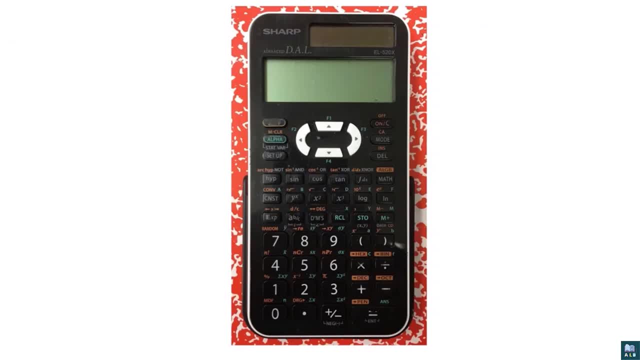 That's your inverse sine. So if you notice up above there, I've got sine to the negative one. That's your inverse sine sine. Now I've got this second function. you see, it's been worn out because I use it quite a lot. 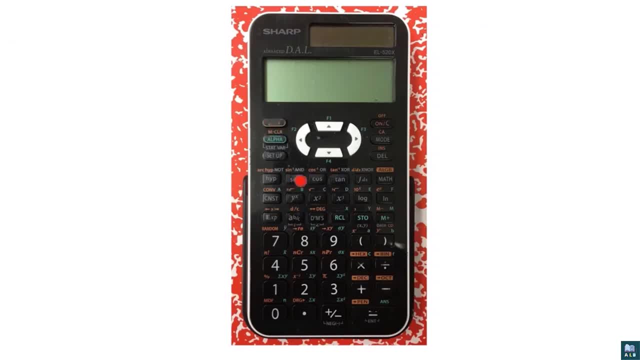 that's like your shift key, so you press second function inverse sine, 0.8- or, depending what your calculator is, it might be 0.8- second function inverse sine. Every calculator is different, so you'll have to get used to it on your own, but that should get you the answer that you're looking for. 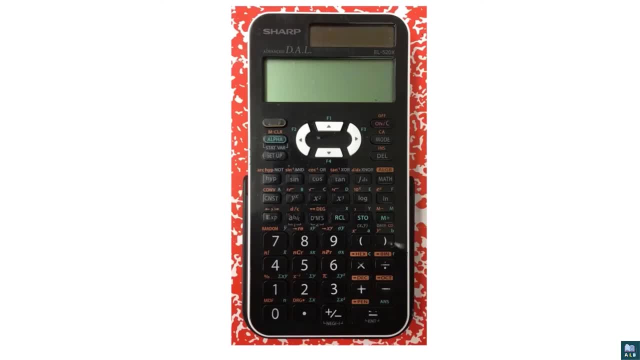 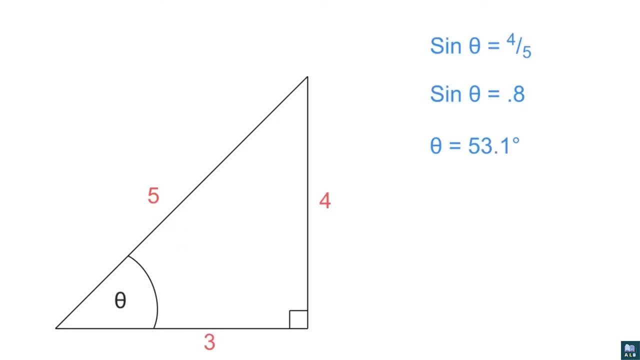 that will get rid of the sine. so inverse sine 0.8 will give you the angle, which is 53.1 degrees. So there you go. we solved the angle. we have solved theta using sine, which is our opposite over our hypotenuse. Now we're going to use the other functions as well. we're going to 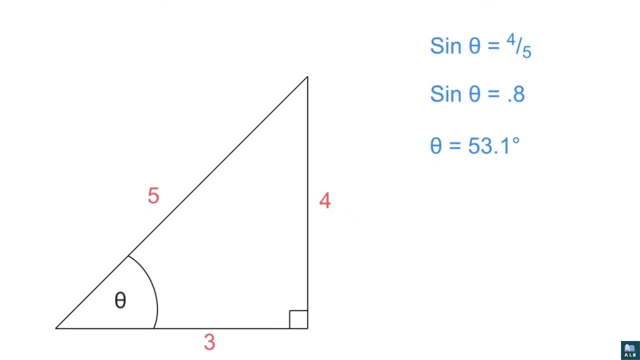 use cosine and we're going to use tangent and hopefully this angle should work out the same using different ratios. So let's take a look Using cosine of theta. same idea. all we have to do is take 3 divided by 5, because we're going to use cosine of theta, So we're going to use cosine. 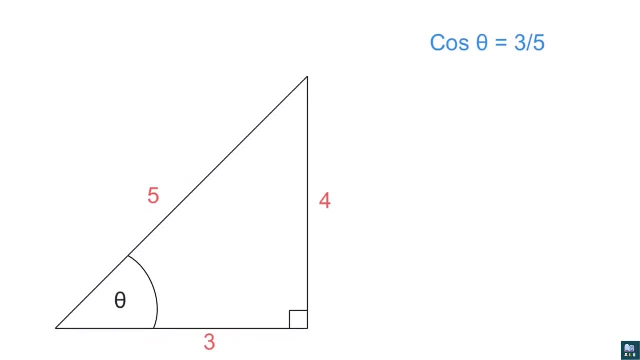 because cosine is adjacent over hypotenuse. So we take 3 divided by 5 and that equals 0.6. so the cosine of theta is equal to 0.6 and again using our calculator, we want to get rid of the cosine. so 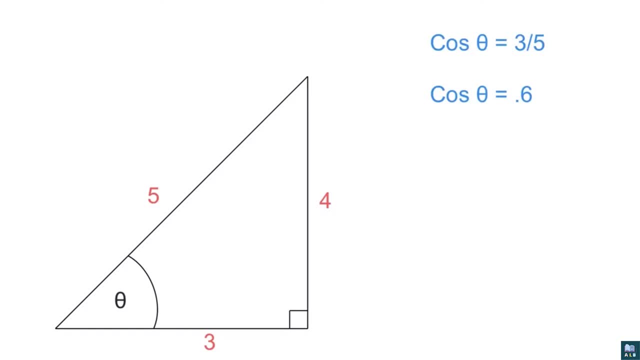 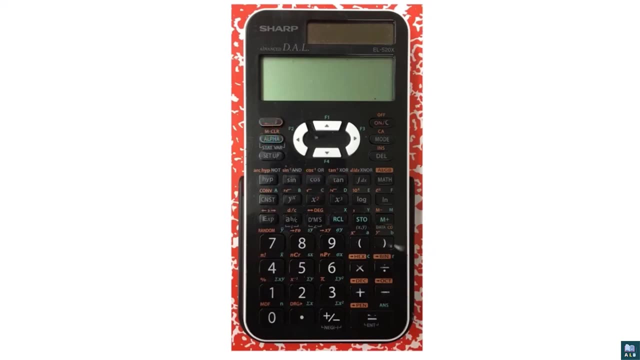 we're going to inverse cosine, that. Let's take a look at that one. So, just as we had before, we're just going to take the second function and we're going to use cosine. so it'll be a second function which gets you that inverse cosine. So we're going to use cosine of theta and we're going to use 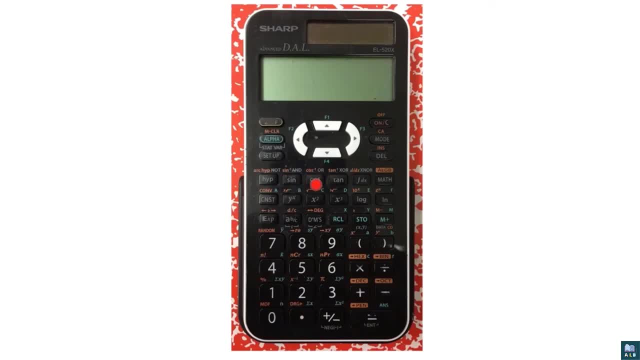 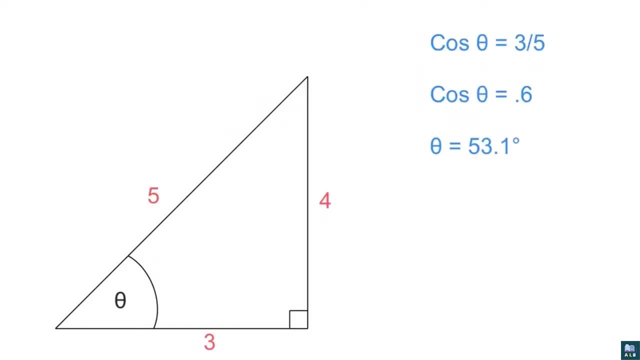 cosine of theta. So again, we'll point in 0.6, second function, inverse cos, to get our answer. or perhaps, depending on your calculator, it's inverse cos 0.6.. Any way you look at it, we're going to get an angle of 53.1 degrees. So we have determined using sine that we can get 53.1 degrees. We've 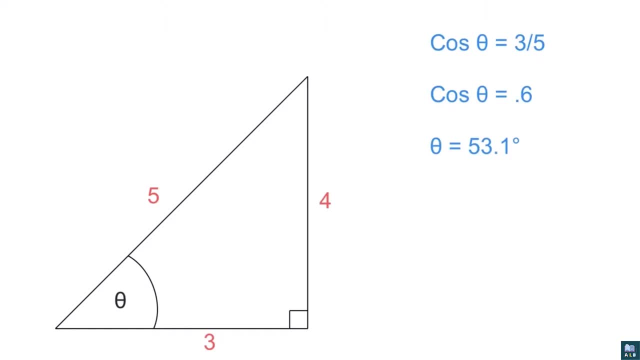 now used cosine. that leaves us with tangent. Let's take a peek at that one. Using tangent, we use the formula TOA. Tangent of theta is equal to 4 over 3, opposite over adjacent. So the tangent of theta- let's turn that into a number- is going to equal 1.33. and again we 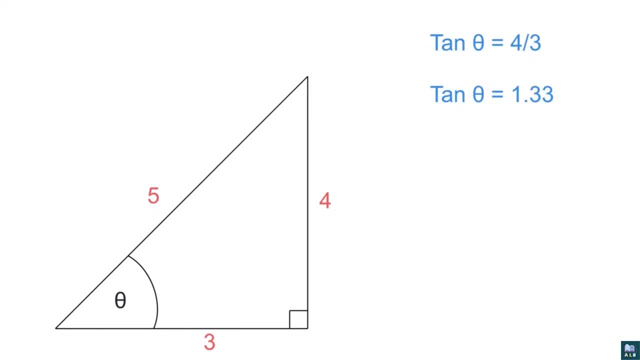 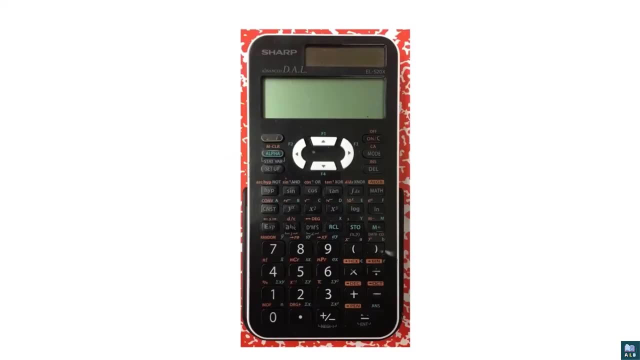 want to get rid of the tan, so we have to inverse tan. that out of there. So let's take a look at our calculator one last time. I'm going to open up my calculator in here and press: inverse tan. 1.33 equals, or you're. 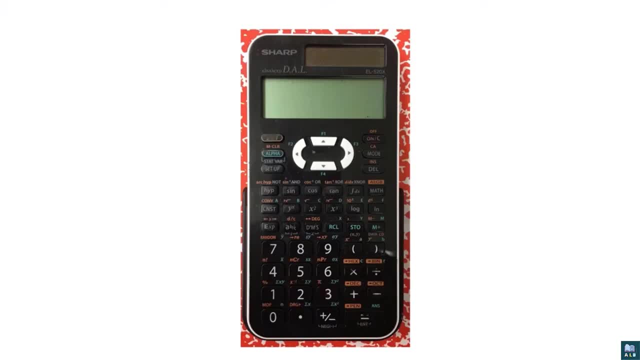 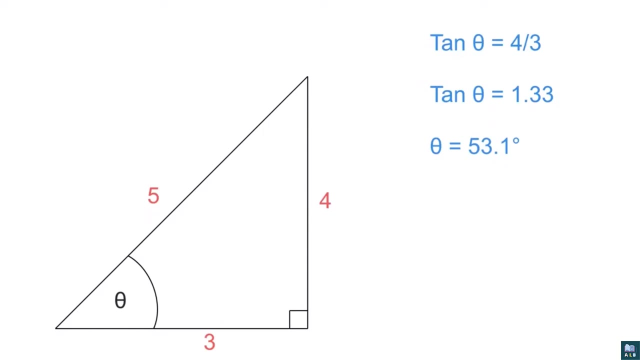 going to put 1.33 inverse tan, depending totally on your calculator, And you should get your angle, which we're hoping is going to be 53.1 degrees, aren't we? Let's take a look? Well, what do you know – it is 53.1 degrees. So there you go. We've determined using any of these. 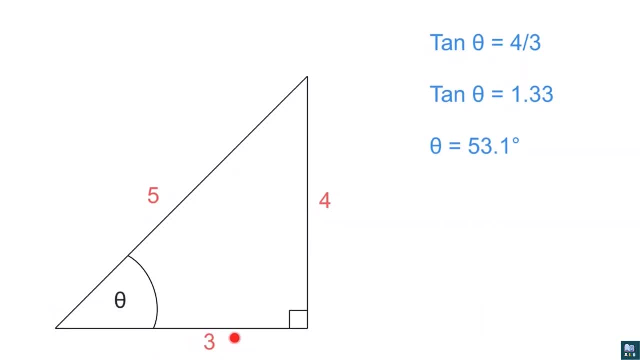 three sides, wwwscienceflagedu or under anotherelvecom, We leave the след crossed with our clothes down. that way we're able to always be in and out of the foundation and I can see if it's sine which is opposite over hypotenuse, cosine which is adjacent over hypotenuse. 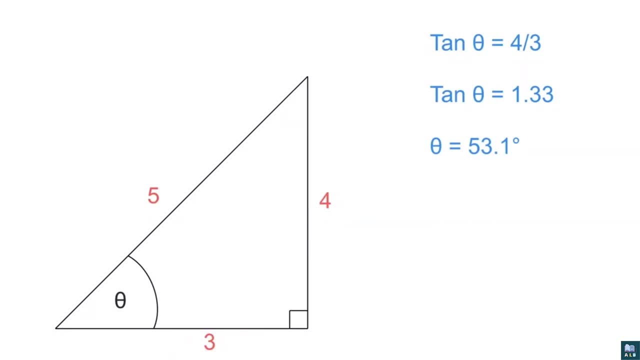 or tangent, which is opposite over adjacent. Using those fun trig functions, we can use it to determine the angle, And that's what we're doing with this one. Now, what we're going to do in the next video is determine what to do when you've got just an angle and a side. How do we work that out? Hopefully this was. 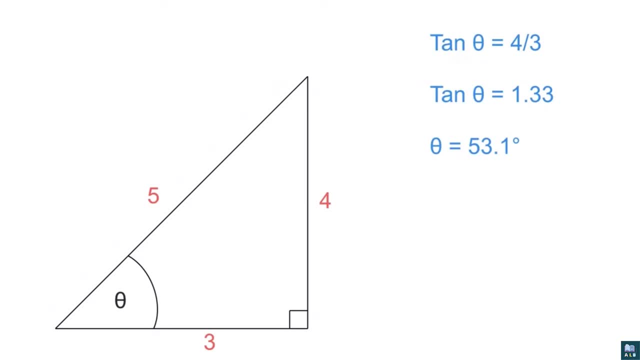 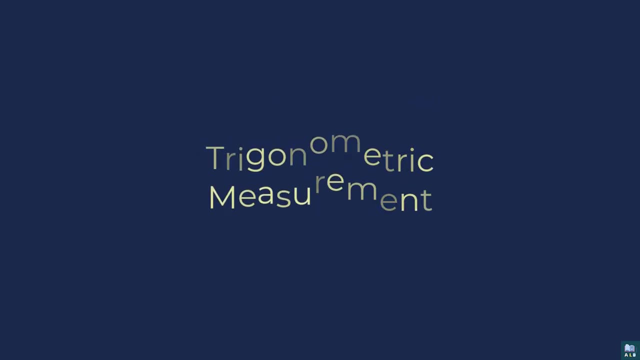 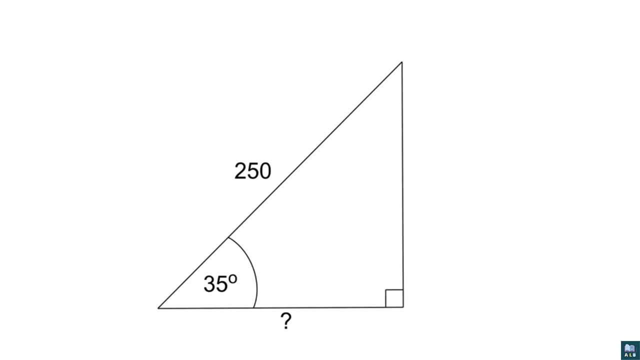 helpful. If you have any questions at all, please leave a comment in the comment section and we'll see you in the next one. In this video, part two of trigonometry, we are going to determine how to figure out the sizes of the sides. these guys here- using nothing but a side and an. 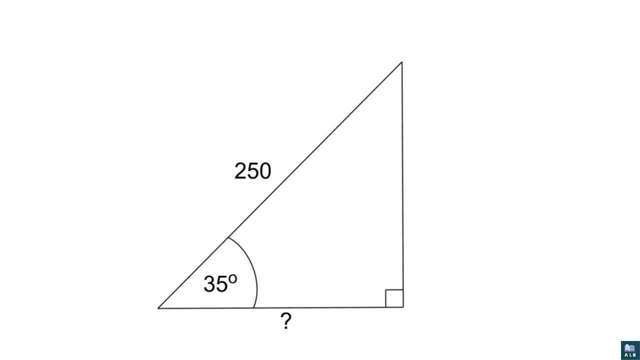 angle. So in this example, we're going to have 35 degrees for a designated angle and we're going to have 250, whatever for our hypotenuse And we're going to try to determine what this adjacent side is. So if we have 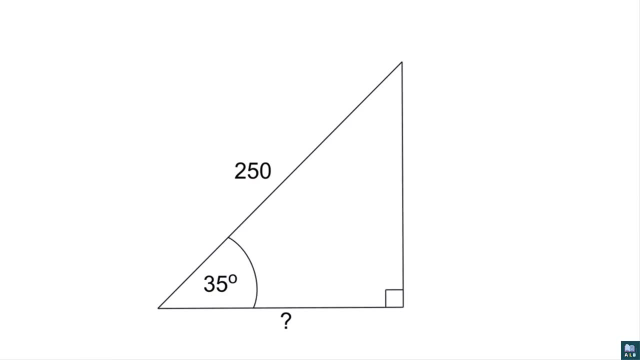 adjacent, we have hypotenuse and we have an angle. we should be able to remember from our last video that we're going to use cosine because we have adjacent over hypotenuse, but we don't know what this is. So let's plug some numbers in, we'll. 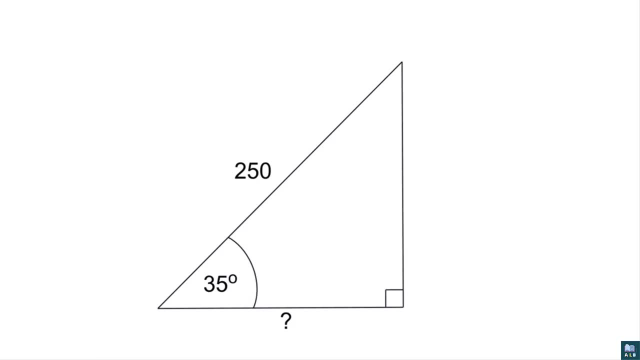 work up the formula and see what happens. Let's remember that the cos is equal to adjacent over hypotenuse. Let's start out with plugging the numbers that we know. So we know that the cos is equal to the corner of absolute and absolute mitre. Let's also plug in the numbers according to our legs, so this: 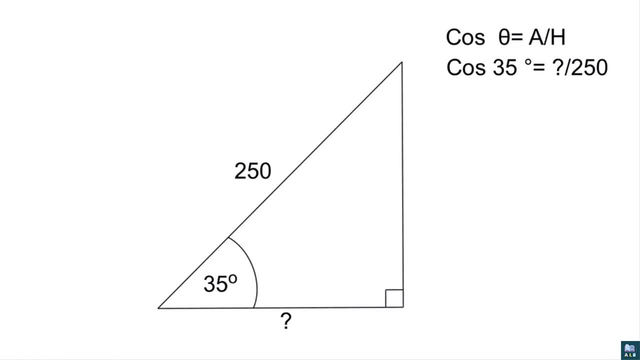 theta is also. the cos of 35 degrees is equal to the- we don't know- over 250. let's transpose that now. however, before we transpose, let's just get rid of this cos 35. what we're going to do is just punch it in your calculator and if you need to remember how to use the calculator, watch the last. 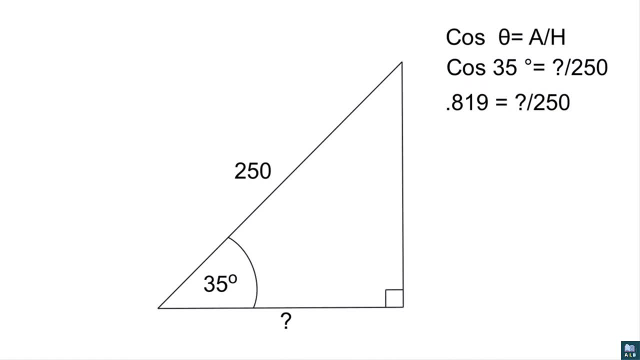 video. but instead of using our inverse cos we're just going to go, cos hit the cos button 35 degrees and that gives us 0.819. 0.819 is equal to, we don't know, over 250. now we can start the transposition. 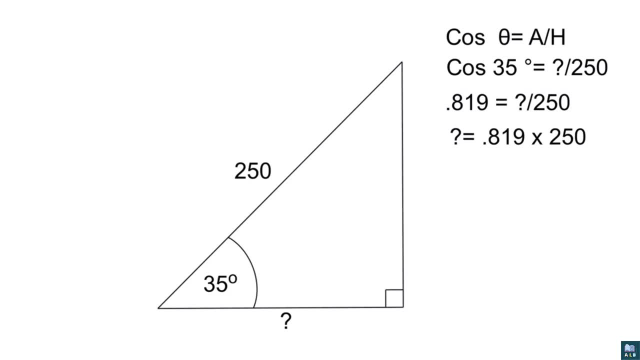 we flip it around, so we're going to divide this guy out of here. we're going to move this guy over to here, so we end up with: the unknown is equal to 0.819 times 250, because all we have to do is cross, multiply and we're going to get an answer of 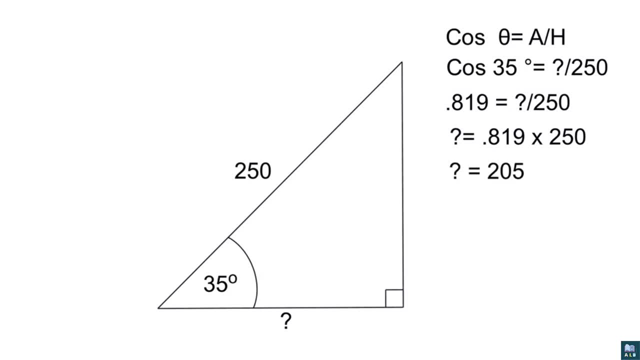 205.. so that's not that bad. let's get that written in there. so basically, it is just like using what we did in the last video, except now we just need to know what this side is. so we're using the same formula, we just have our unknown over. 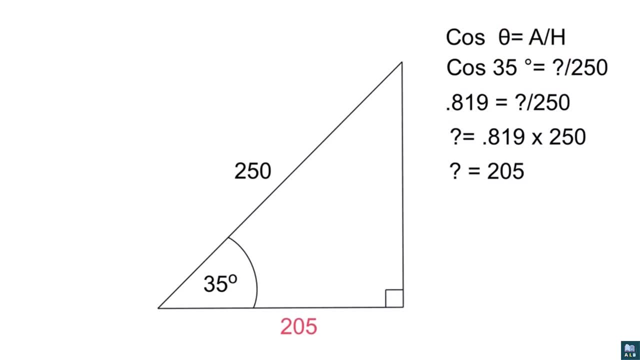 here as opposed to our unknown- being the angle. so that's using cos. so we're going to walk through all three as we did in the last one. so that's cos. for our next one, we're going to use our total Overall и we're looking at this here. we have an opposite and we have adjacent and an angle. so to me it looks were going to use tangent. Tangent of theta is equal to opposite over adjacent, so let's plug the numbers in that we have. the tangent of 48 degrees is equal to 300 over what the tangent of 48 degrees is equal to 3.5.what 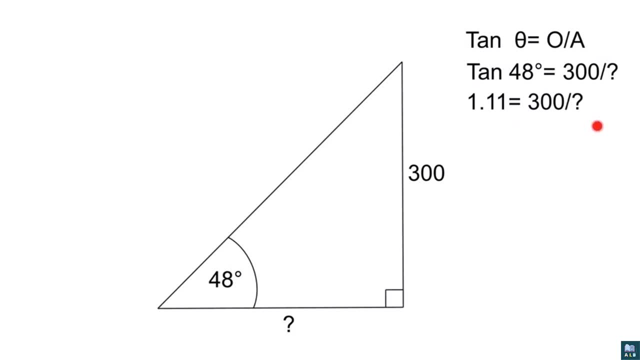 calculator and we get 1.11 is equal to 300 over what? so we transpose that now we've got 1.11 times we don't know is equal to 300. so we'd have to make one more step in our transposition, which tells us that our unknown factor here, or 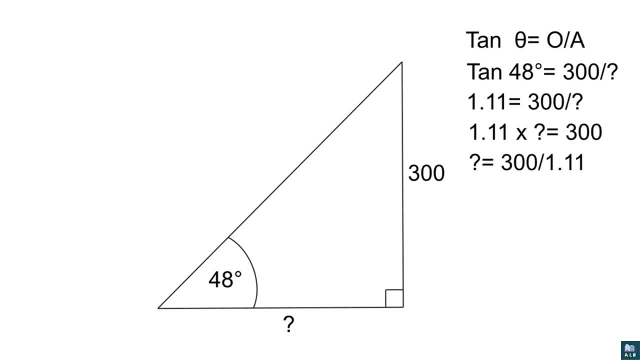 the what is equal to 300 divided by 1.11, and we get our value of 270. so let's get that plugged in there. so there you have it again, just using tangent with what we know. now it leaves us with one more. we've already done cosine and we've 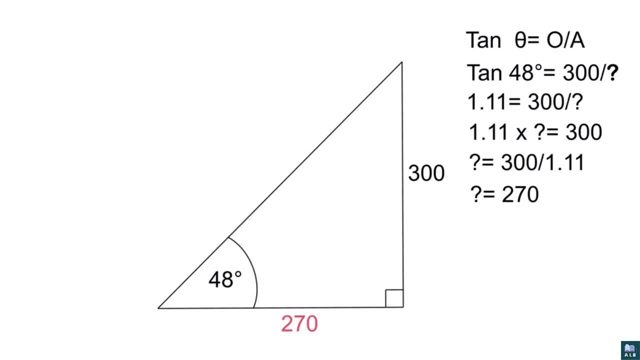 already done tangent. so let's mix it up a bit and we're gonna finish strong with sine. now you can tell we're going to use sine because we have an unknown here. we have our hypotenuse. so we have our opposite side, which is unknown: our hypotenuse. 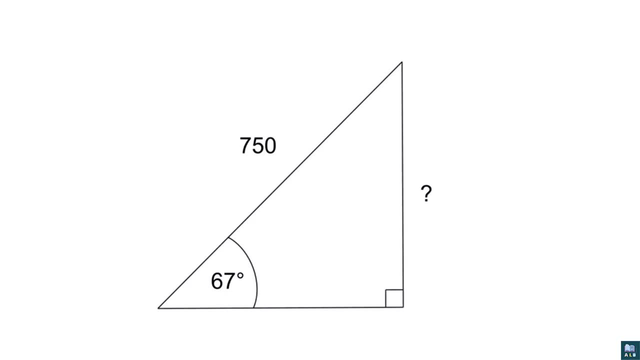 which is 750, and our angle, which is 67 degrees. so our sine is equal to opposite over hypotenuse, which is shown right here. the sine of theta is equal to opposite over hypotenuse. let's plug in the numbers so we can see what we're. 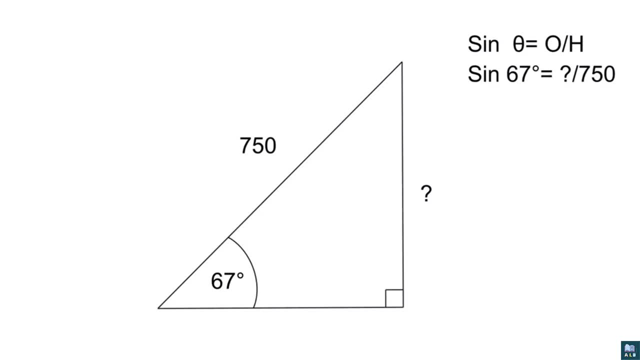 working with the sine of 67 degrees, which is theta here, is equal to. we don't know what that is, but we do know that the hypotenuse is 750. so let's get rid of the sine of 67. punch sine 67 into your calculator. 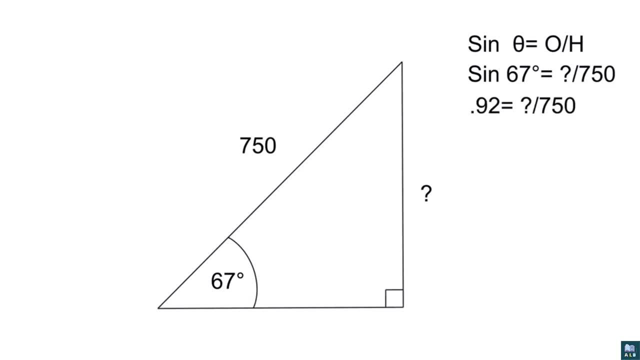 and then you get: .92 is equal to the unknown divided by 750, and we can just cross multiply. let's take a look what's next. using cross multiplication, we end up with our unknown as equal to influencers. their unknown is equal to 0.92 times 750, which gives us a numerical value of 690.. 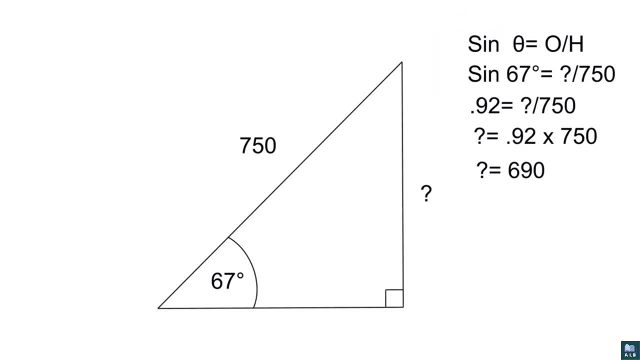 So let's punch that into our side of triangle. here And there you have it: 690.. So we've gone through them all. We've gone through tangent, using a side and an angle. We've gone through cosine, using a side and an angle. 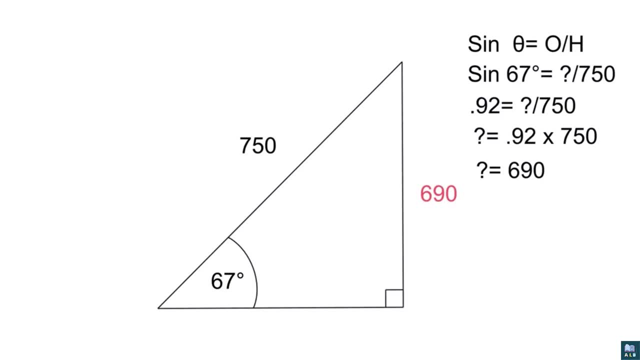 And now we've gone through sine using a side and an angle. It's not that hard once you have the concept of that. sine is equal to opposite over hypotenuse, cosine is adjacent over hypotenuse and tangent is opposite over adjacent. 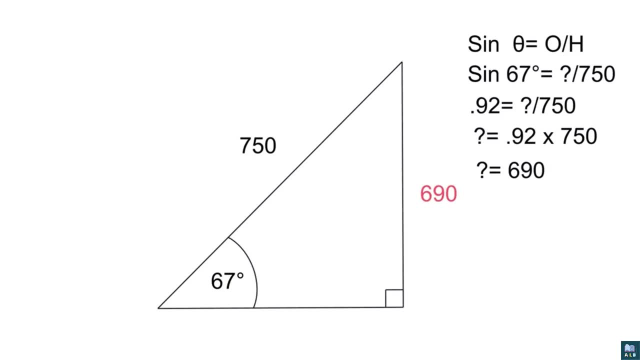 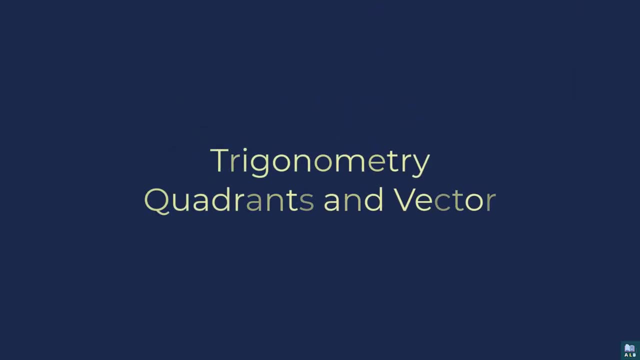 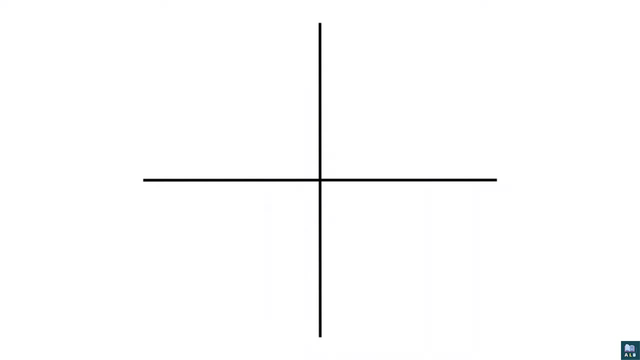 Once you've got that down, if you go through these couple videos a couple times and some worksheets, you should have no problem at all. This video is going to be the first in a series of videos I'm going to do on adding vectors. Now, in order to properly add vectors- and the easiest way to add vectors, I find, is using the quadrant system- 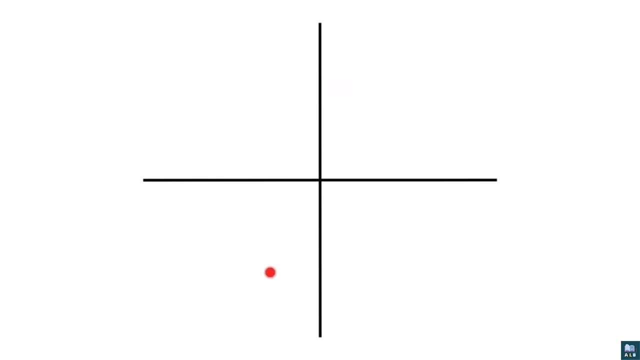 Now, what I mean by quadrant system is this thing: here I've got this guy divided into four spots, hence the quadrant. Now I'm just going to go over some characteristics of the quadrant, and in the next video I'll start talking about converting from one form to another, and the next one will be another form to another, and then we'll get into 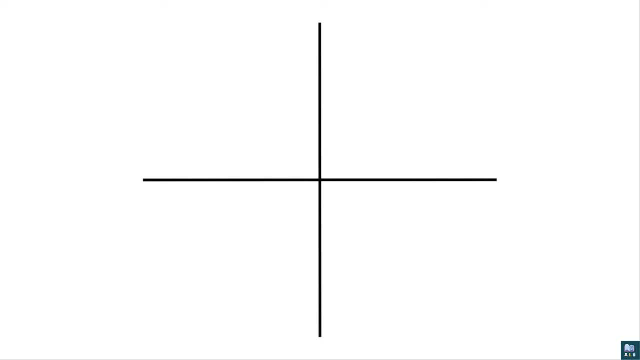 the addition of the vectors. Now in our quadrant system we have four quadrants. We have one, two, three, four and they are labeled as such. Here I've got quadrant number one, quadrant number two, quadrant number three and quadrant number four. 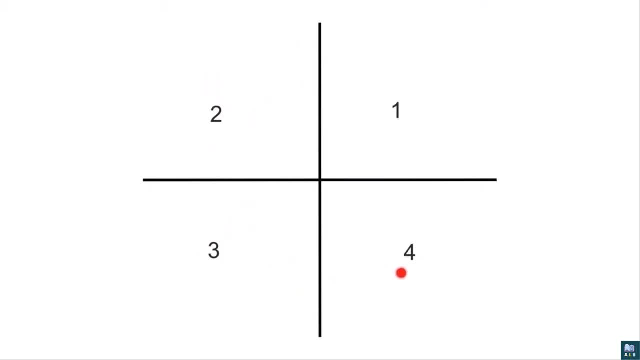 Now we have them kind of backwards. They go in a counterclockwise direction. you'll see here, That's because vectors, when they rotate- and we'll talk about this later on- but they rotate in a counterclockwise direction. 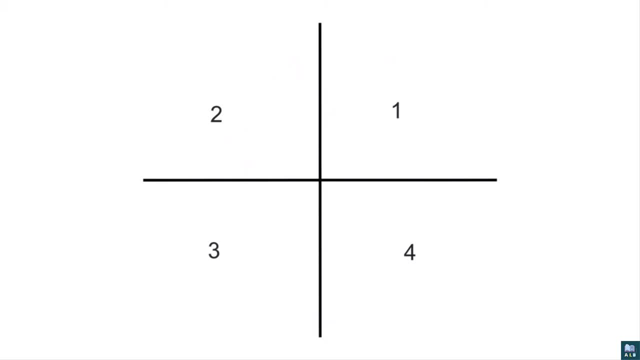 So I'm going to label them this way: One, two, three, four. Now, when we're dealing with these quadrants, it's very important that we understand the angles that we're dealing with. Now I'm going to start right here and say that this point, right here, is angle zero. Up here is angle 90.. 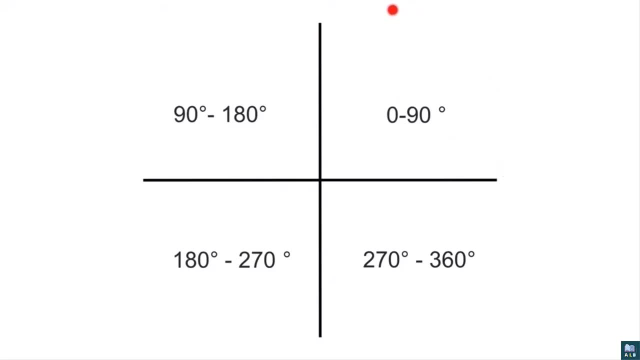 So in quadrant one we are dealing with angles between zero and 90 degrees. Quadrant two is between 90 and 180.. So again, quadrant two is going to deal with angles between 180 and 90,, so 90 and 180, and then so on, and so on. 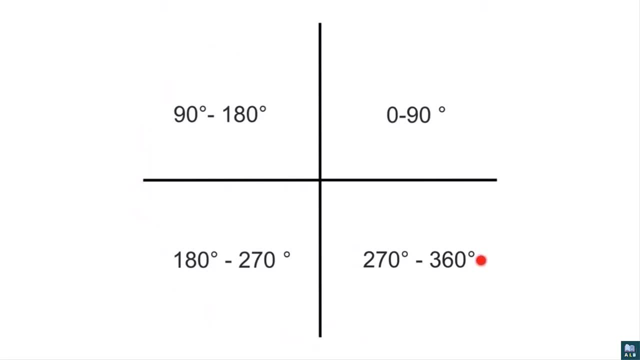 We've got 180 and 270.. 270 and 360.. So that's the angles. That's going to be very, very important as we move on in this Now, as we're looking at the system here, it's very important that we understand how the polarities work in each quadrant. 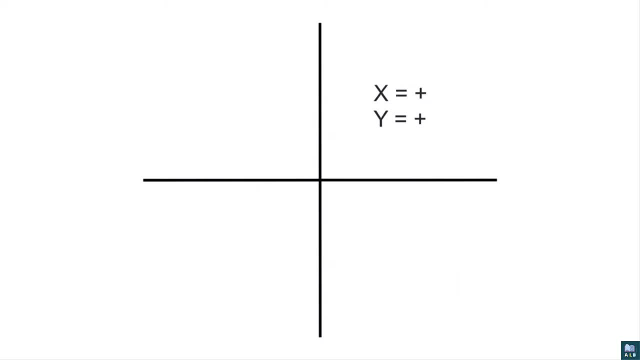 Now, just as a quick refresher for this quadrant system, we're going to talk about the x and the y-axis. The x-axis is anything that runs this way horizontally. The y-axis is anything that runs vertically. We have a part here where the energy is going to go to the left and then to the right. 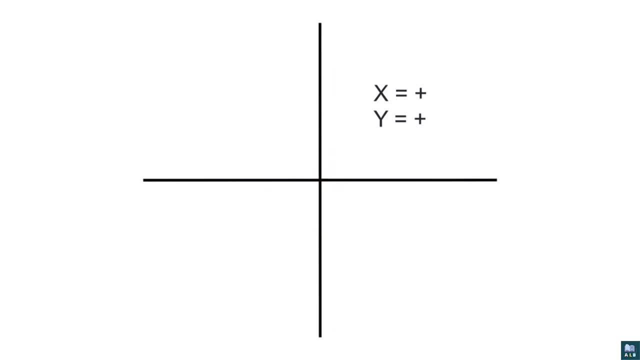 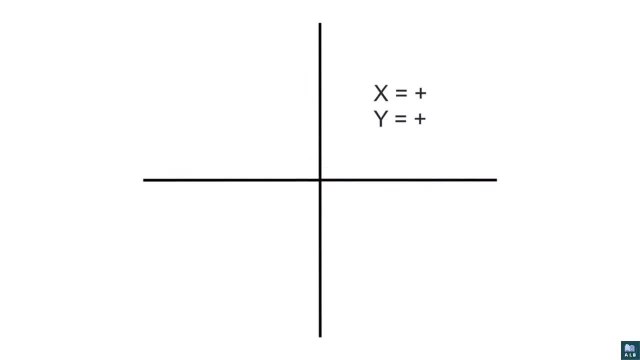 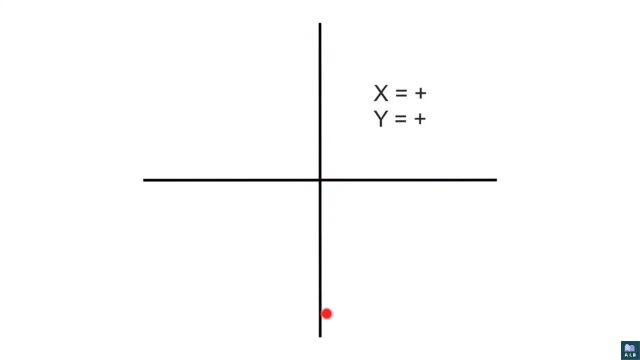 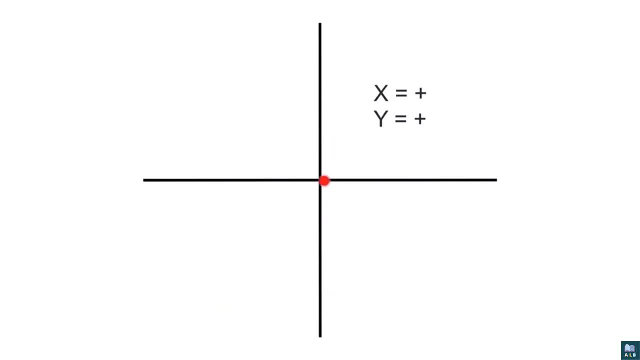 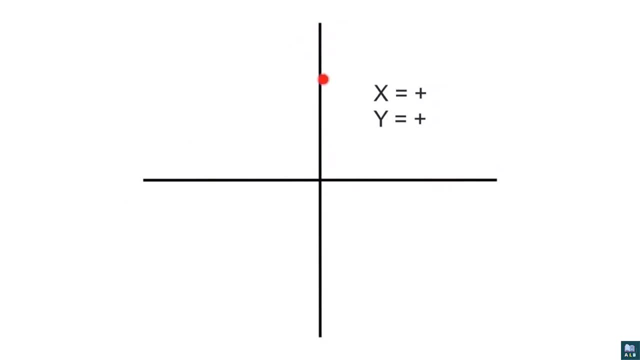 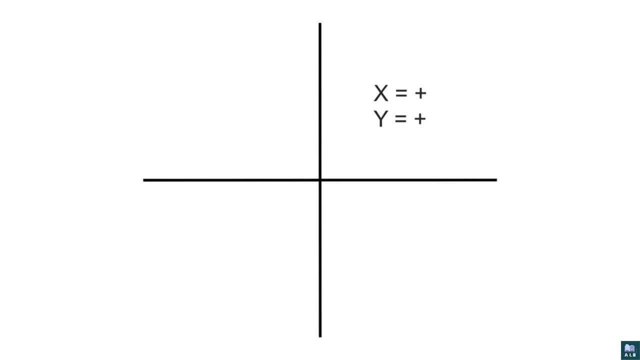 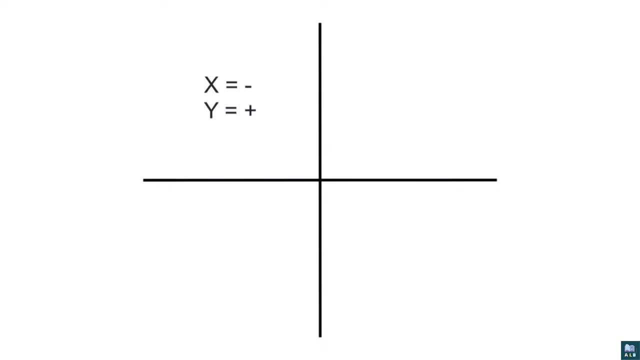 The y-axis is anything that runs vertically. Now, if we look at quadrant number 2, we're dealing with a quadrant where the x is negative. It's on the left-hand side of the point of origin, but the y is still above the point. 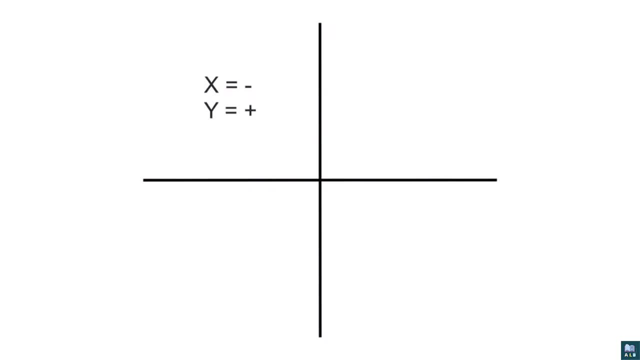 of origin. So our x is negative and our y is positive. In quadrant number 3, my x is negative because we are to the left and my y is below the point of origin. So x is negative, y is negative. and to sum things up in not sum things up to be talking about quadrant number- 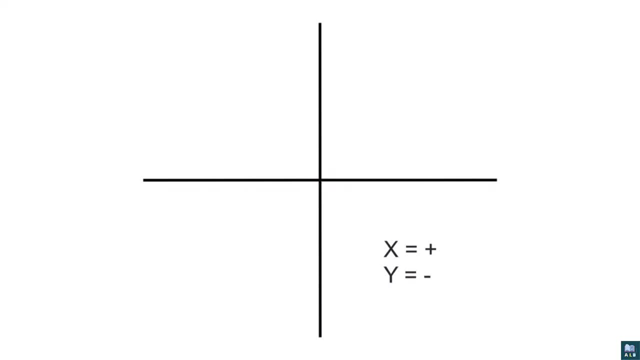 four, i see that i am to the right, so my x is positive, but i'm still below the point of origin, so my y is negative. so that's how we work out the quadrant system. again, we have four quadrants: one, two, three, four. this quadrant is anywhere between 0, 90, 90 and 180, 180, 270, 270, 360, and then we have 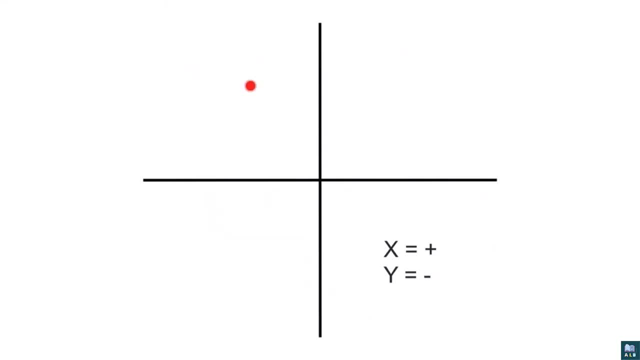 our polarities- positive, positive. this one here is negative, positive, negative, negative, positive, negative- and that's how the quadrant system works. in the next video, we'll discuss what happens when we throw some numbers at these things. we're going to start converting from what's called polar to. 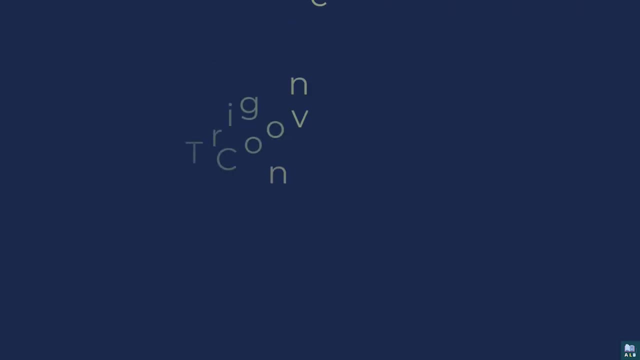 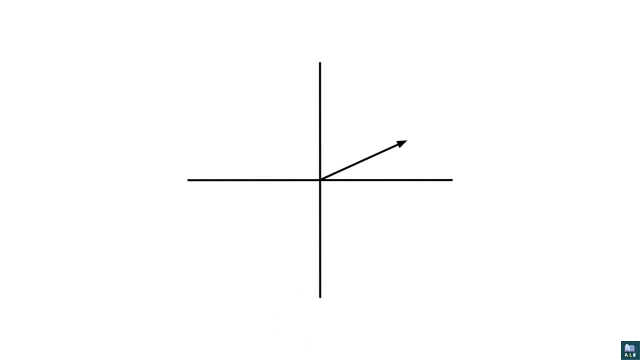 rectangular. in my last video, we discussed what the quadrant system was. now i'm going to get down to brass tacks and show you why it's important now. the reason why we use quadrants is because of vectors, and a vector is something that contains magnitude. so how large it is, and direction, which way is it? 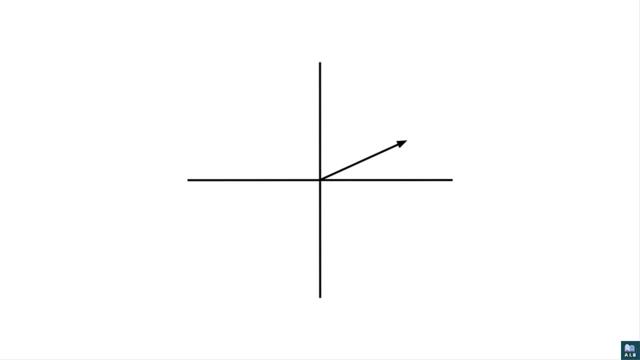 heading. a vector can show up in any of the four quadrants: one, two, three or four. in this case, this vector here is whatever size, this is at whatever angle, which is the direction in quadrant one. so we're going to get down to brass tacks and show you why it's important now, the reason why we use. 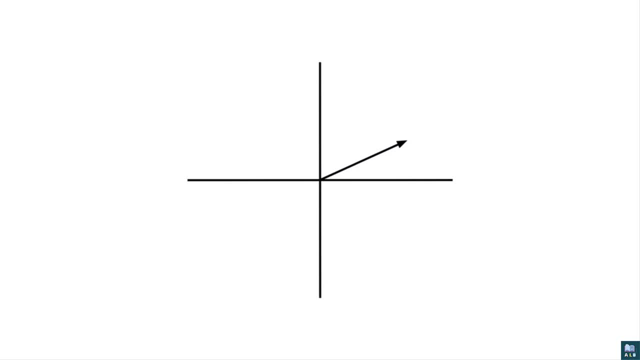 there's two ways that we can look at vectors. we can look at them in what's called polar form or rectangular form. in this video i'm going to go through about converting from a polar vector to rectangular coordinates. so let's take a look here now. in this example here i'm saying: 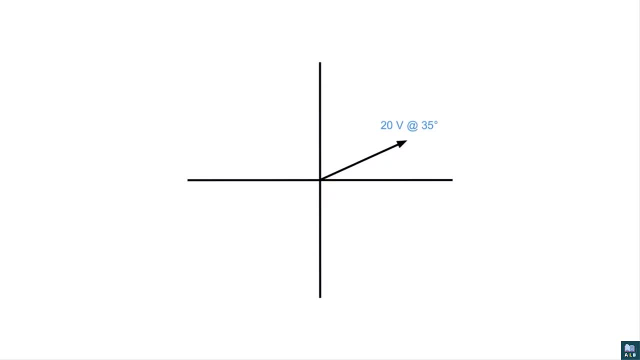 that this vector is 20 volts and it's heading off at 35 degrees. the way that we've expressed this vector is in what is known as polar form, so it's giving you its magnitude and at what angle it's going at. so magnitude and direction. now, when we want to add vectors, however, 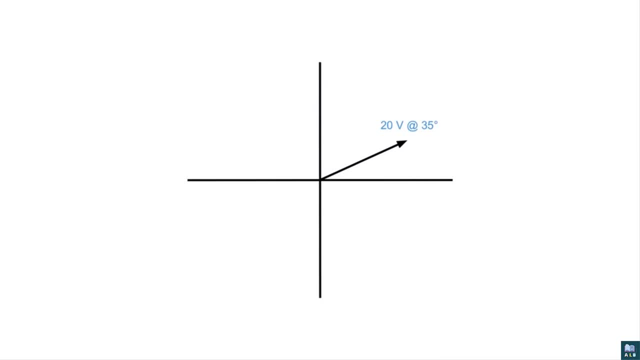 it would be a lot easier for us to kind of break these guys down into an x and a y coordinate. and we can do that now because you guys have been given the power of trigonometry. we know that this guy here is 20 back- sorry, 20 volts. so that's my hypotenuse if i want to figure out what my x is. 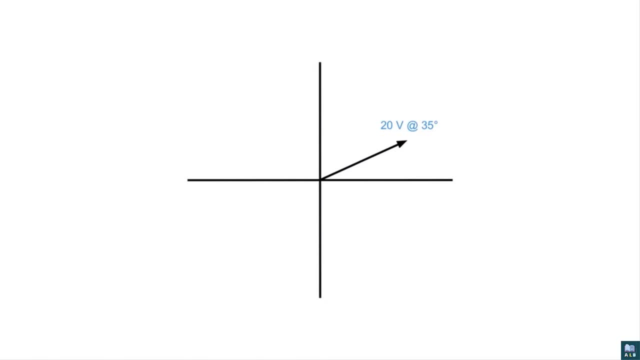 i can figure out this guy here and this guy here. that makes us a right triangle. so i can use trigonometry to figure out what the x is and what the y is, and what the y is and what the y is, and this is a very important part of trigonometry. now, if i want to figure out what the bottom is here, 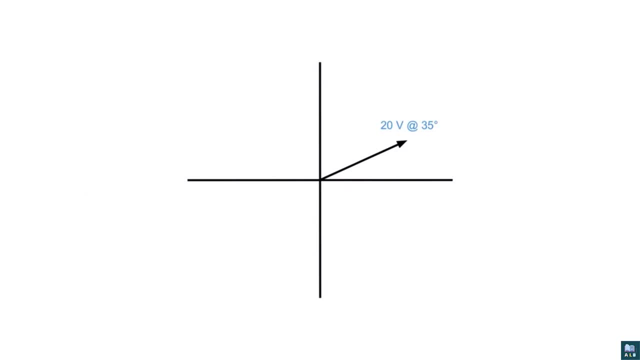 the adjacent to this angle, i'm going to use cos. when i want to figure out what my y is, i'm going to use sine, because i've got cos is adjacent over hypotenuse and sine is opposite over hypotenuse. so let's kind of break this down here: using cos, i can figure out what my x coordinates are. 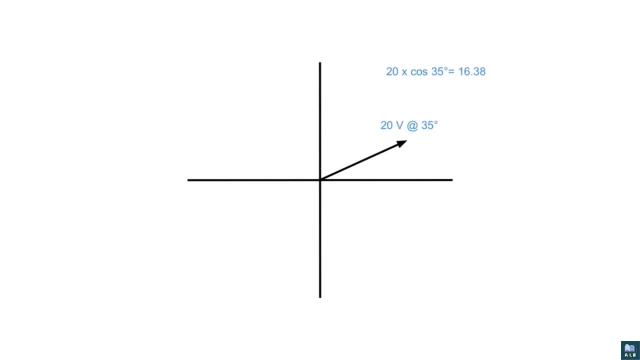 i can take 20 volts times the cos of 35 degrees and i get that my x is going to work out to be be 16.38, or 16.4, if you want to get funky with the rounding. Now I'm going to take the same thing. 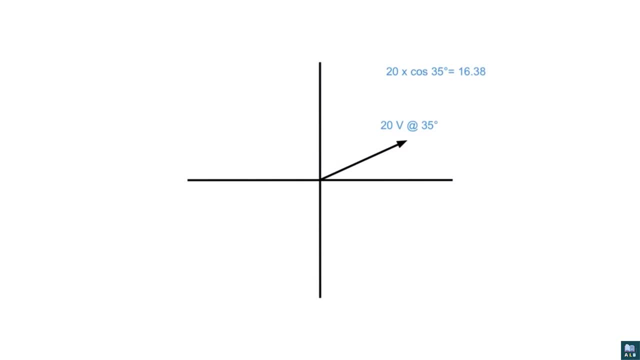 I'm going to go 20 times the sine of 35 degrees. It's just a little shortcut instead of having to transpose all the time, And I'm going to get my y coordinate. Actually, I've got that 16.4 there. 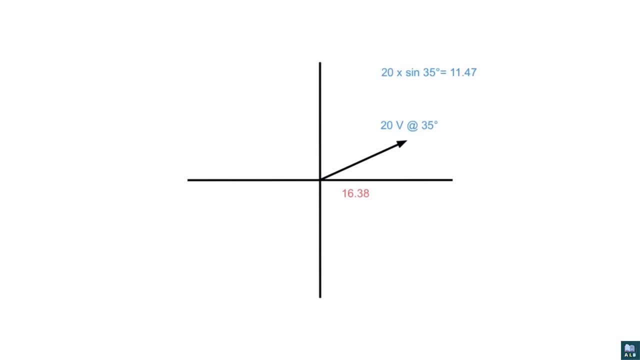 Now my y is 20 times sine. 35 is 11.47, which is going to be this side right here. So I've got that punched in there. So basically now I have my x and my y, which is the same thing. 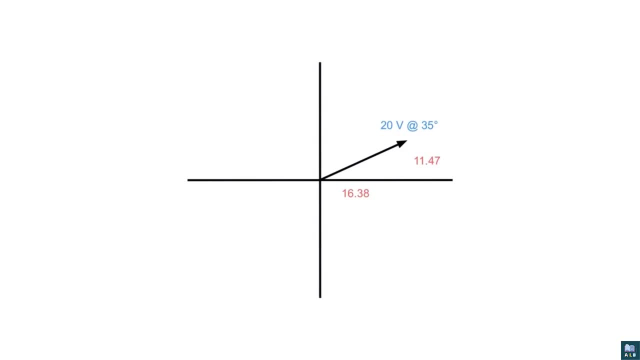 as this here. So this form, 20 volts at 35 degrees, is your polar form, Your x being 16.4 and your y being 11.5, that is what's known as rectangular, And we differentiate our y from our x by throwing. 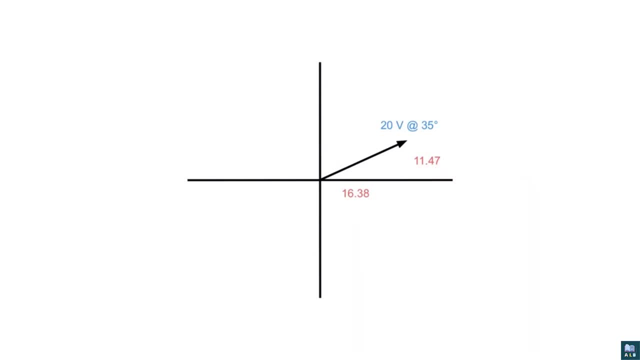 a little j in front of it And you can go to my notes in my lesson plans that I'll have and it'll explain, give you a little explanation, Explanation as to why we use j. So there we go. We've got 16.4 or 16.38 and j 1147.. That is the. 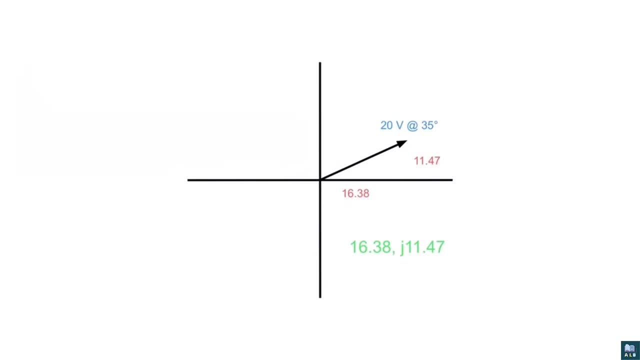 rectangular form: This guy and this guy, they are identical. So that's in quadrant one. Now, in quadrant one, remember that it's both positive x and positive y. What happens when we end up in quadrant number two? Boom here we got 60 volts, heading at 150 degrees. So we know that in 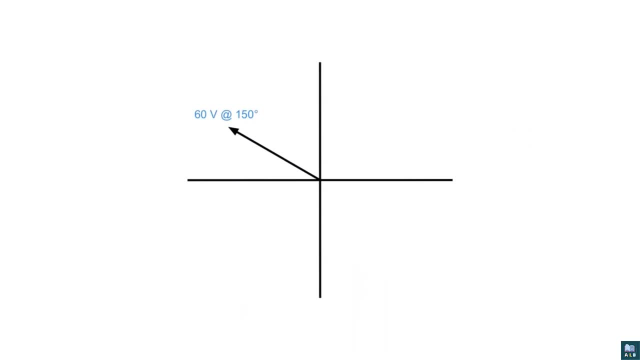 quadrant two, we have a vector of 0 and 90.. Quadrant two is between 90 and 180.. So that's going to throw this vector into quadrant number two. Now the same thing is going to go here. All we have to do is go 60. 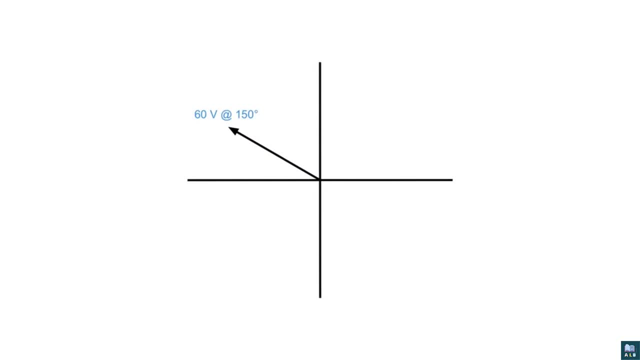 times the cos of 150 is going to give me my x, and 60 times the sine of 150 is going to give me my y. 60 times the cos of 30 degrees gives me 51.96 for the x size. Now let's take a quick look at this before I go on. I've got negative 51.96.. That's negative because I've got my 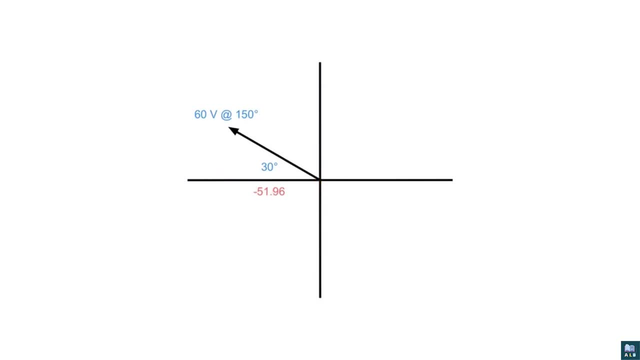 point of origin here, and on the x it's negative- remember from my last video. So that's very important. If you forget that, you're going to screw yourself over. when it comes to adding vectors, Do not forget the polarity. Now, if I take 60 times the sine of 30 degrees, I end up with my y being 30. Now it is above the x axis, right, I'm. 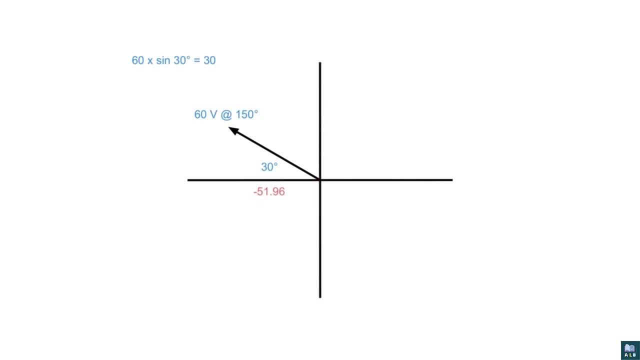 still in this positive sense here. So I could say that this guy is going to be positive 30.. So now I can say that my coordinates, my rectangular expression of this vector, is going to be negative 51.96 and j 30.. 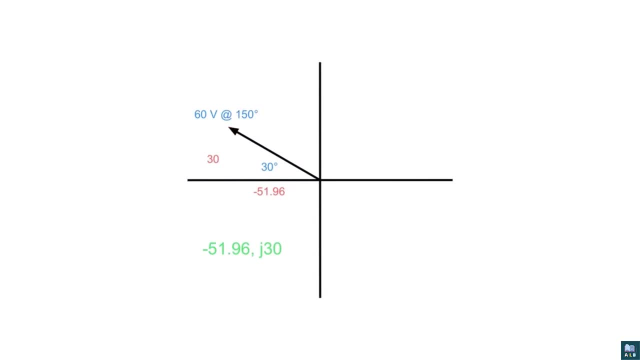 So that's giving us our second quadrant. Now, why don't we fool around? We've got two more quadrants to go through. Why don't we just do them and get them over with, and that way you guys can see how it works for every single quadrant? 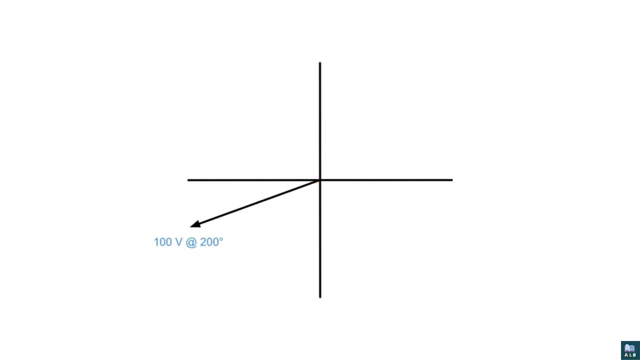 Now in quadrant number three, I've got 100 volts, which is the size, the magnitude, and 200 degrees, which definitely throws me in the third quadrant, because anything between 180 and 270 gives me quadrant number three. Again, I'm going to go 100 times the cos of 200 degrees gives me my x, which 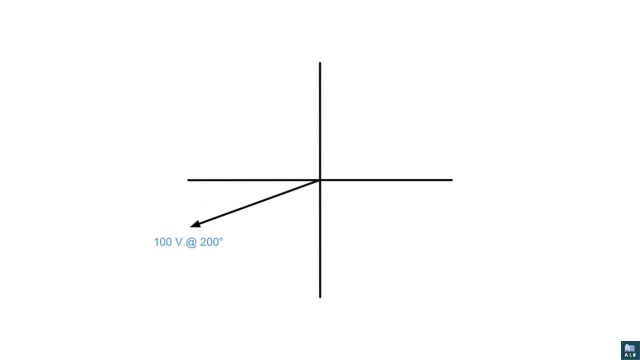 is going to be negative And in this case my y is also going to be negative. So 100 times the cos of 20 gives me negative 93.97.. See, I've got that negative in front of it. 100 times the sine of 20 gives me 34.2.. 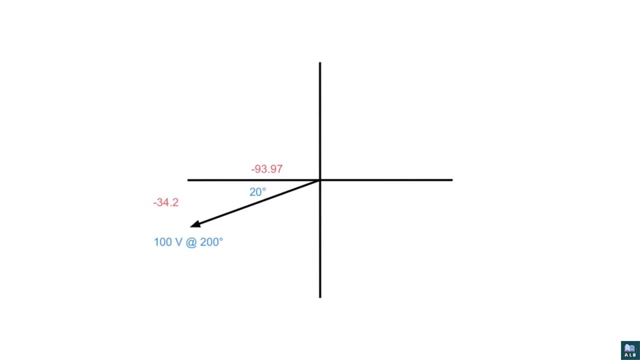 But I put down negative 34.2 down there And then I can express this as negative 93.97 and negative j or j negative 34.2.. So again, this is polar, this is rectangular, And let's finish it up here. in quadrant number four I got 90 volts at 320 degrees. 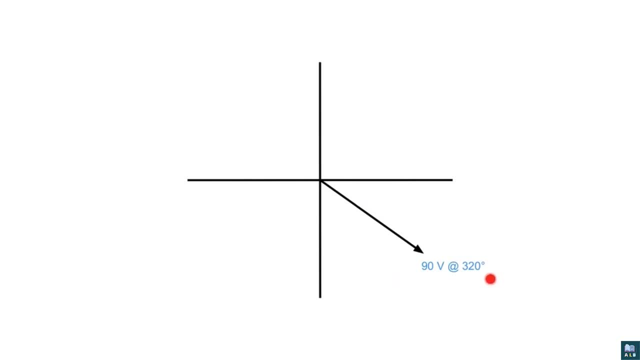 So again, same thing: 90 times the cos of 320 degrees is going to give me a positive x, And then my y, however, is going to be negative. So again, I cannot stress enough the importance of those polarities. 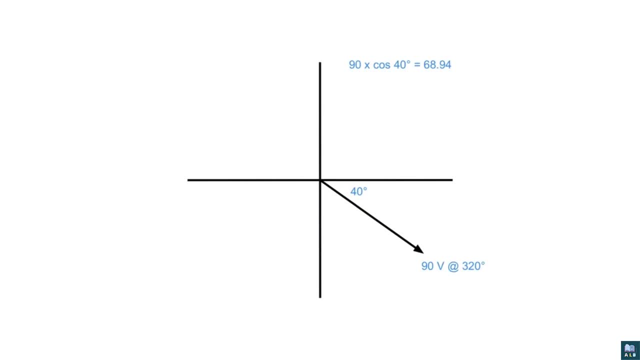 So 90 times the cos of 40 degrees gives me 68.94 right here. So that's going to be a positive 60.97.. So I've got that at 3.98.. And that's going to be negative 90 times the cos of 320 degrees, which is going to give me a negative number. 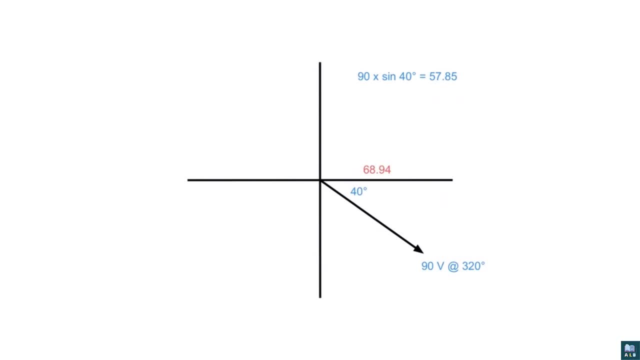 So I've got that as 57.85, which is right there. so that will be a negative 57.85.. And there we have it. If I've got my polar form, which is 90 volts at 320 degrees, and these two guys here can be expressed as: 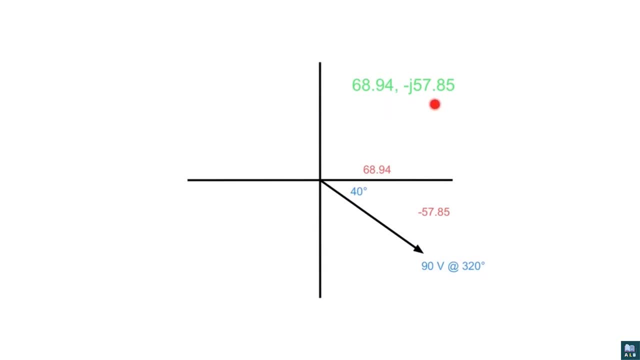 68.94,, negative j 57.85, and that's how you convert rectangular or sorry polar to rectangular. Polar is when you've got the magnitude and the direction, so you've got your angle and the size, and rectangular is your x and your y coordinates, and remember that our y is 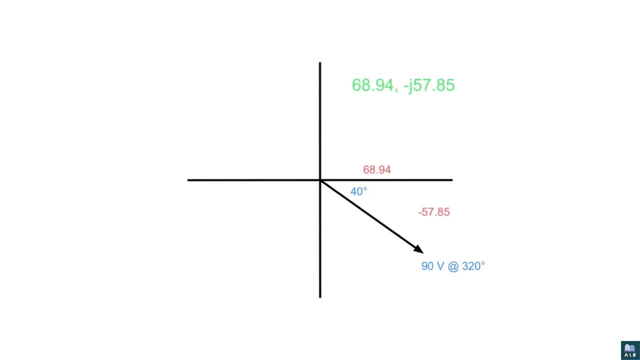 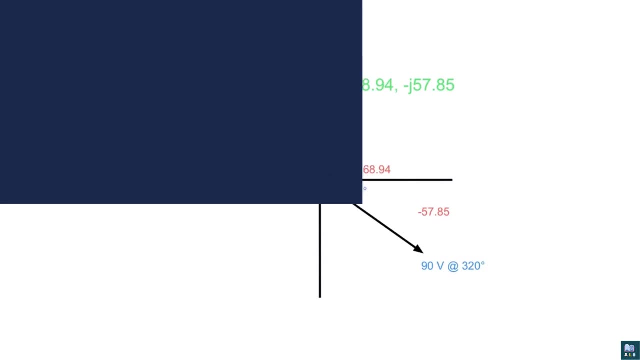 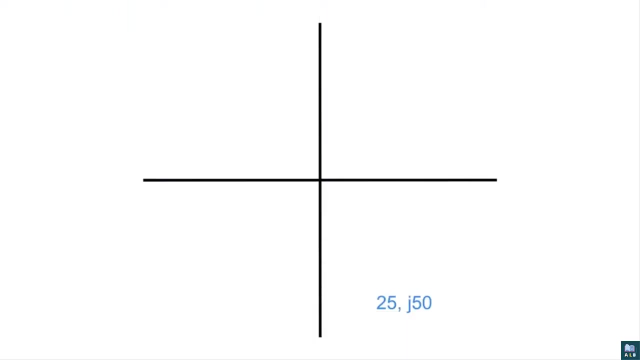 always preceded with a j, just so we can tell the difference between the two. and also, again, I know I keep saying it, but do not forget your polarity. In this video, we're going to be going over how to convert from rectangular form which. 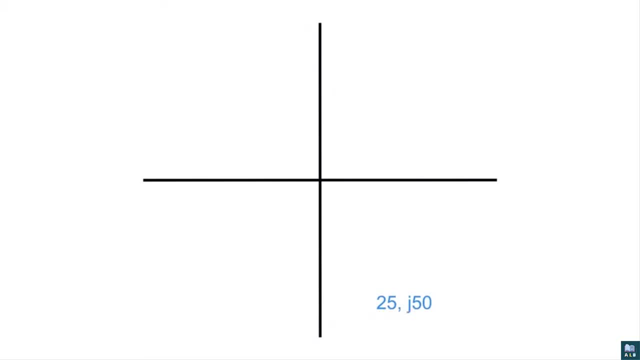 is when we break it down to an x and a y coordinate. when we take a vector and we work out what its x is and its y, we're going to take the rectangular form and convert it to polar. So what we're going to do here is we're going to start out with this vector right here. 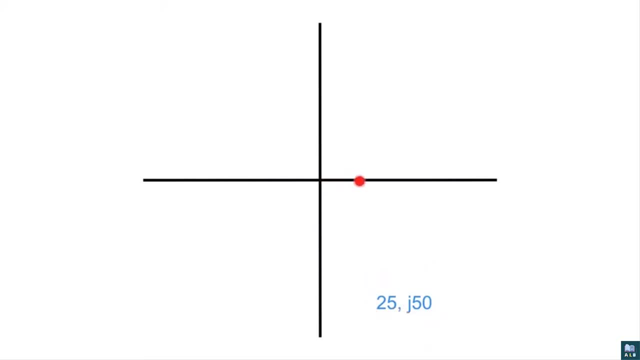 We've got an x of 25 and a j of 50, which means that we've got an x of 25 and a j of 50 here. It means we're going to be in quadrant number one. So let's throw some numbers at that. throw some picture up here, just so we get our head. 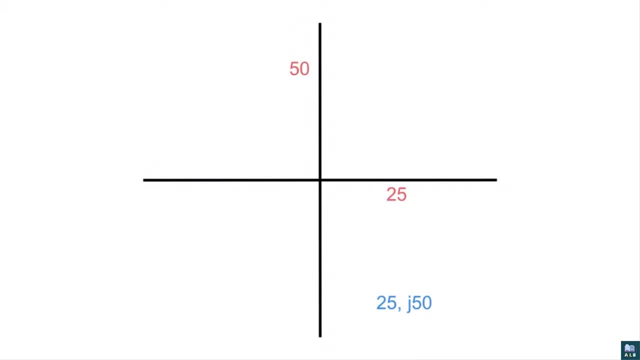 wrapped around it. So I've got 25 on my x and I've got 50 on my y, so let's just draw the vector in. So I've got 25 here and 50 here. So now what we need to do is figure out what our hypotenuse is. 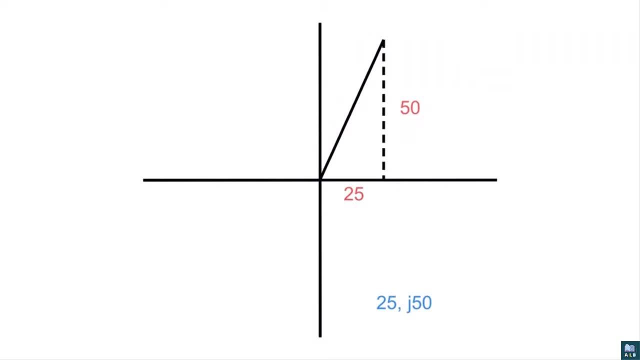 Okay, What our hypotenuse is going to be, and this is our resultant, which is the first part. This is the magnitude that we're looking for when we're talking about the polar form, as we learned in our last video. So we're going to go: 25 squared plus 50 squared gives me the square root of 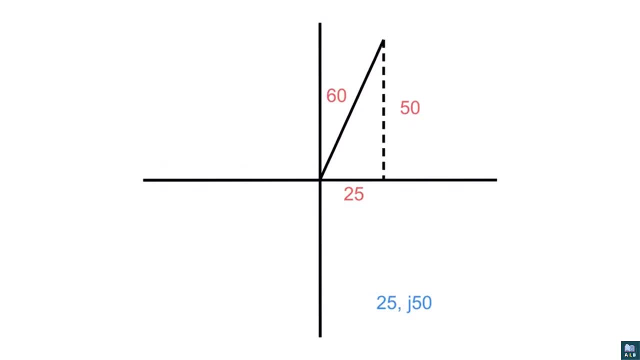 We end up with a resultant of 60.. So that is the magnitude. Now we need to figure out what direction it's heading in, and that would be our angle. So what I'm going to do is use cos I'm going to go: 25 divided by 60. 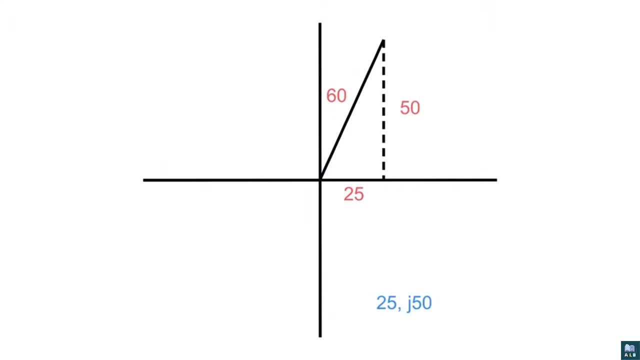 And then I'm going to inverse cos that And if you want to know why I'm doing that, you just need to watch the videos on trigonometry. But I'm taking my adjacent side and my hypotenuse, and adjacent over hypotenuse is the ratio. 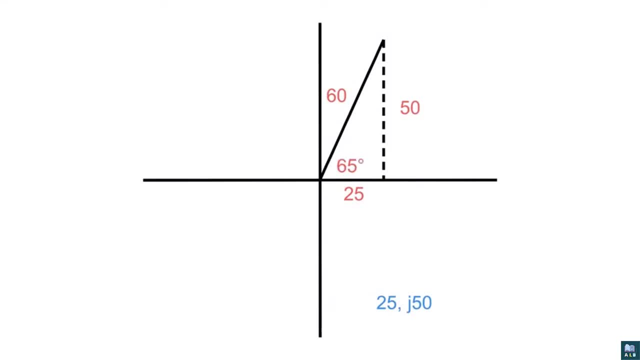 of cosine. So I do that, The cos of 25 divided by 60, inverse cos that I get 65 degrees. So now I've done it, I've figured out that my magnitude is 60. That's my resultant, the hypotenuse. 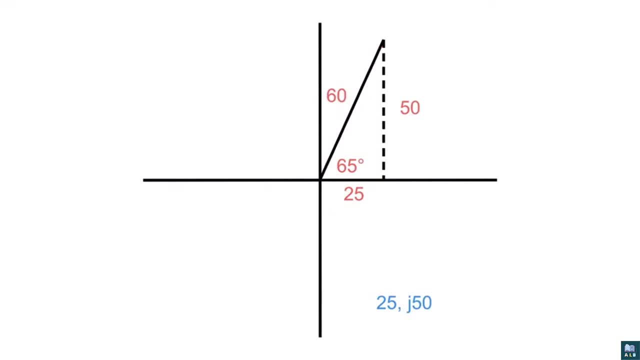 The angle here is 65 degrees And because I'm in quadrant one, which is this quadrant, here again, watch the video on quadrants. it's anywhere between 0 and 90 degrees. I can just easily say that it is 60 at 65 degrees. 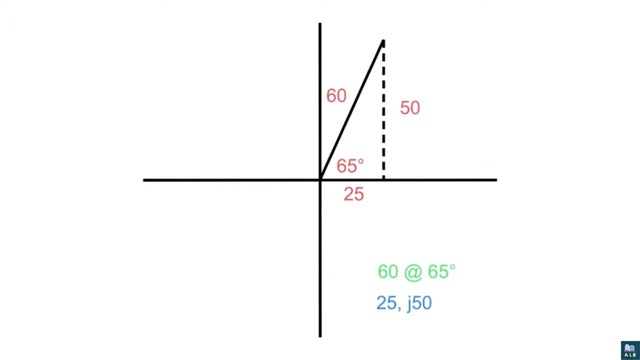 So there you go, We've got 60. at 65 degrees is the polar form of 25j50.. That's in quadrant number one. Let's move around the four quadrants like we've done in the previous videos, and let's 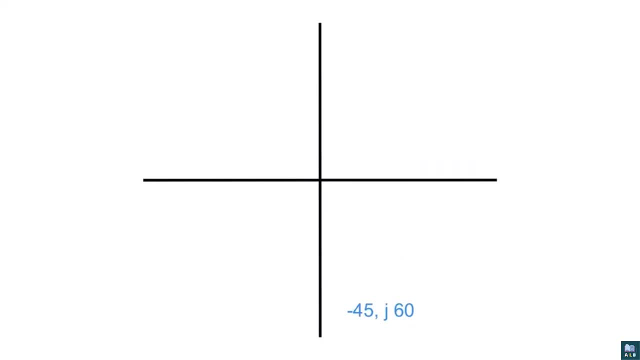 see what happens. So in this example now we've got negative 45, which is negative. 45 is on my x, so it means it's heading this way. 60 means it's heading up, So that puts me in quadrant number two. 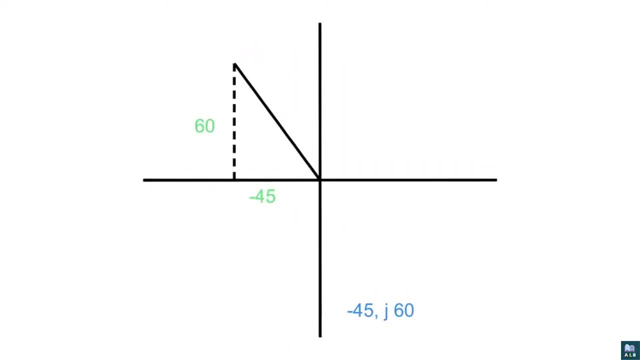 So let's get that started to be drawn up. So I've got negative 45 right here and I've got 60 here Again, through the power of Pythagoras, 45 squared plus 60 squared gives me the square root of 75.. 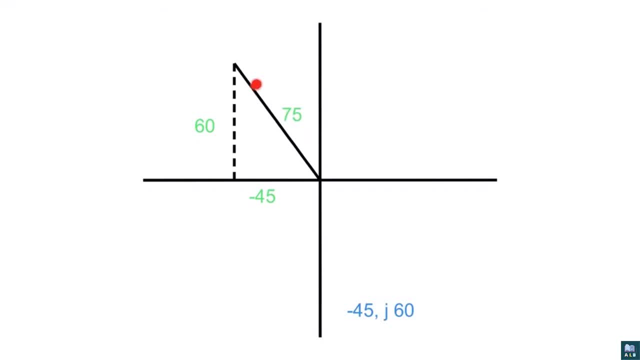 75, again is my resultant, And I'm going to do that. I'm going to do that. Now, what we're going to do is we're going to figure out what the angle is in here, and this part's really important. 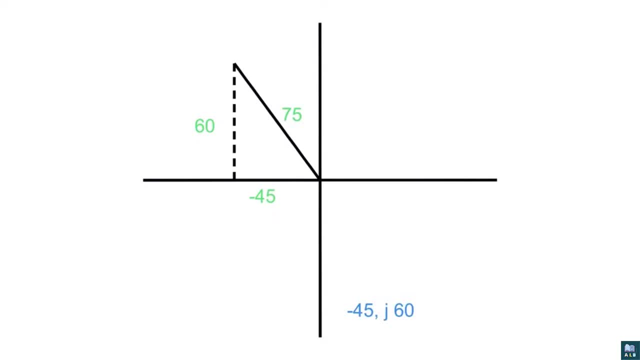 So let's take 45 divided by 75 and inverse cos that and that gives me 53.1 degrees. So now I've got all the sides and the angle here. Now if I was going with polar form I could say 75, but I cannot say at 53.1 degrees because 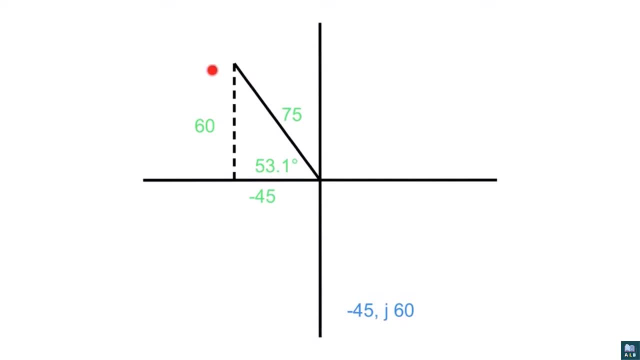 we need to look at which quadrant we are in. We are in quadrant number two, which means that our angle has to be anywhere. It's going to be anywhere between 90 and 180 degrees. Well, we know that this guy here is 53.1 degrees and we're looking at the angle as in reference. 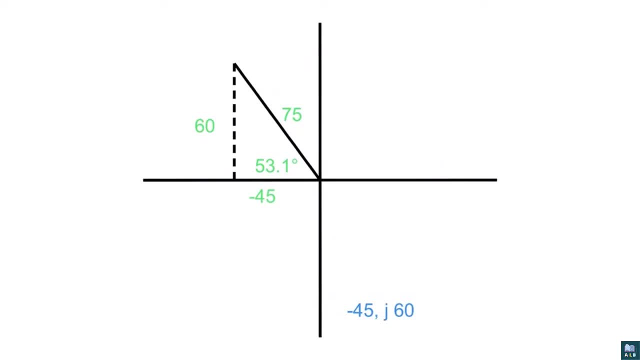 to zero. so we want this angle. So what we're going to do is just take this guy here, 180, minus the 53.1 degrees here to get my actual angle in this quadrant, And I get 129.6 degrees. 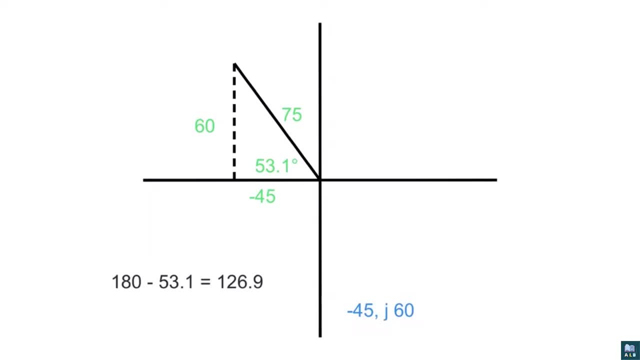 So now I can easily say that this guy here, this negative 45j1, is my actual angle. So now I can easily say that this guy here, this negative 45j1, is my actual angle in this quadrant. So now I can easily say that this guy here, this negative 45j1, is my actual angle in 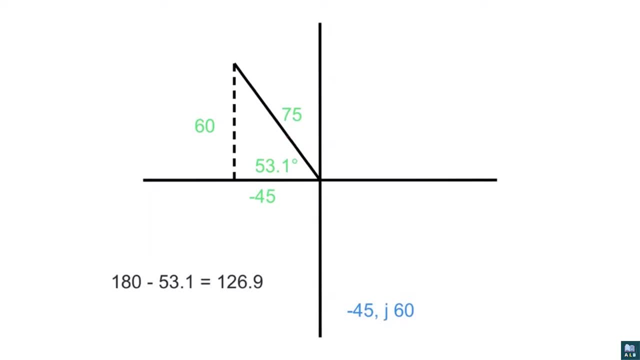 this quadrant. So now I can easily say that this guy here, this negative 45j1, is my actual angle in this quadrant. So let's go to quadrant three. Let's go to quadrant three, So I've got a polar form of 75 degrees at an angle of 126.9 degrees. 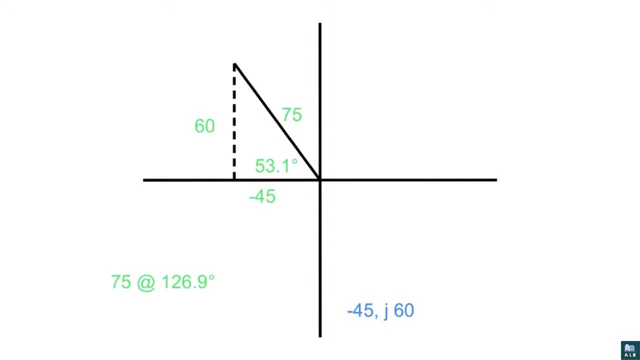 And there you go. that 126.9 tells me we are in quadrant two as well. Let's move it around. Let's go on to quadrant three. So now I have negative 120, negative j40.. So negative 120, negative j40, we know for sure that we are in quadrant number three. 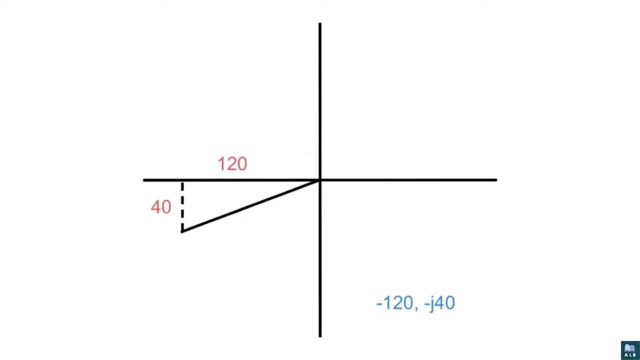 start playing around with this. Get it drawn up here: 120.. So that's the negative. 120 puts me on this side of the X, at the point of origin. 40 is down here. So now I need to figure out what my resultant is, or my hypotenuse, And that works out to be a hypotenuse of 126.5,. 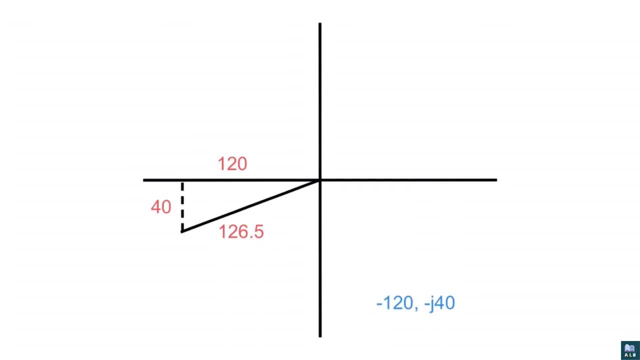 which is my resultant. So again, we're getting there. Now we just need to figure out what this angle is. Again, using cos, I'll go 120 divided by 126.5 and inverse cos, that guy and I get an angle of 18.5 degrees. Now, again, we are in the third quadrant. I can't 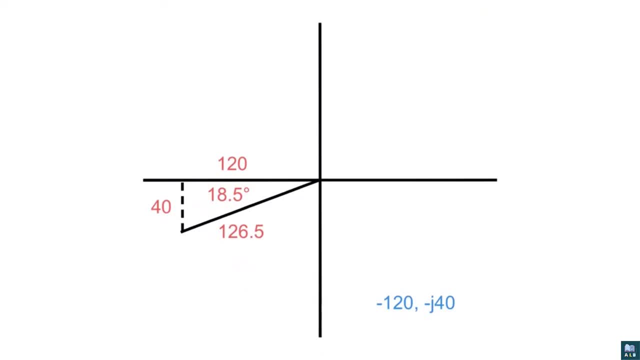 go ahead and say it's 126.5 at 18.5 degrees, because then you think I'm talking about the first quarter. So before in the last one we went 180 minus that angle that we worked out to get the angle. Now we're going to go 180 plus the one. 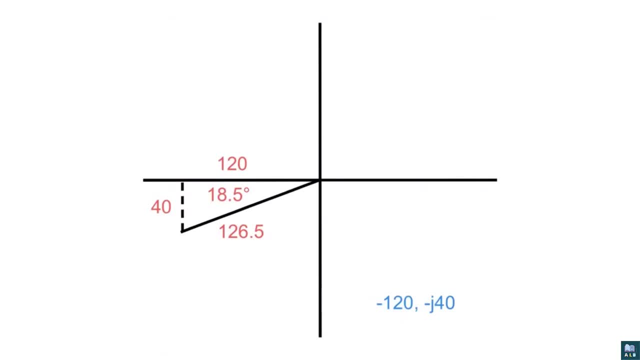 Sorry, the 18.5.. And that will give me my angle, which is 198.5.. So now we can say that our rectangular form, which is negative 120,, negative j, 40, has got a polar form of 126.5. 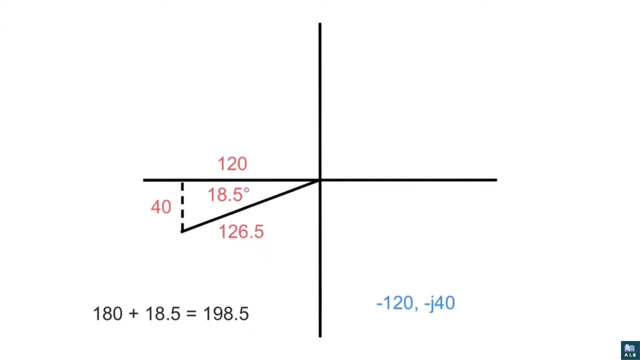 at an angle of 198.5 degrees. There we go. So we've done the first quadrant, we've done the second quadrant, we've done the third quadrant. let's move on to the fourth quadrant: Positive 30. So we're moving this side of the point of origin. negative j: 75 going below. 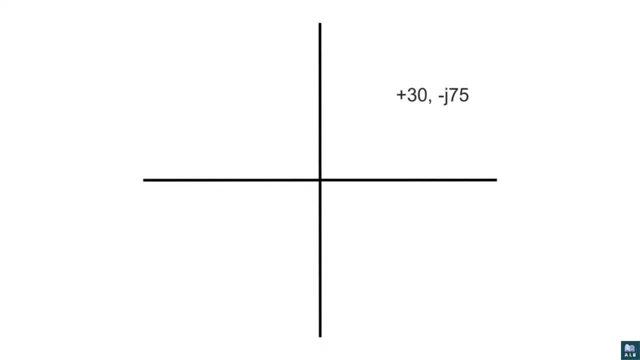 there Again, we are in quadrant number four. So, as we've done before in every single quadrant, all we have to do is draw that in there. get your triangle drawn in: 3075.. Using Pythagoras, we figure out what my resultant is: 80.7.. Now we're going to work out what our angle is. 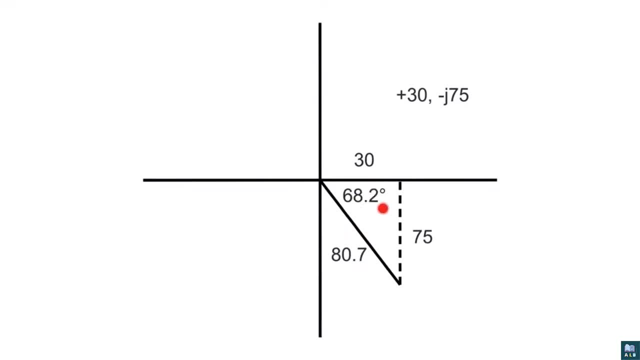 here 68.2 degrees. So now we can say that we've got a resultant of 80.7.. And we know that this little angle in here is 68.2 degrees. Now we said that this angle on this side. 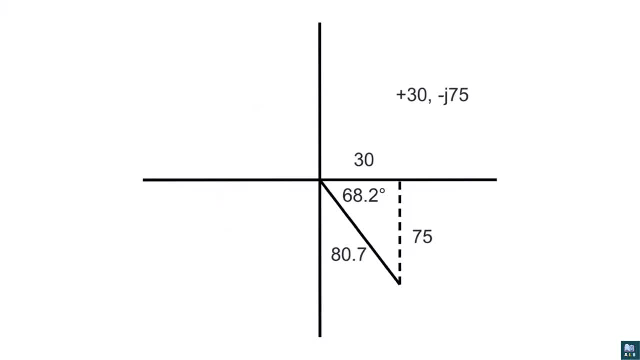 was 180 minus. the angle on this side is 180. Plus we can say that the angle over here is 360 minus and that will give us an angle of 291.8 degrees. So we could say that this guy, 30 and negative j, 75 rectangular, is the same as saying 80.7 at 291.8 degrees. But 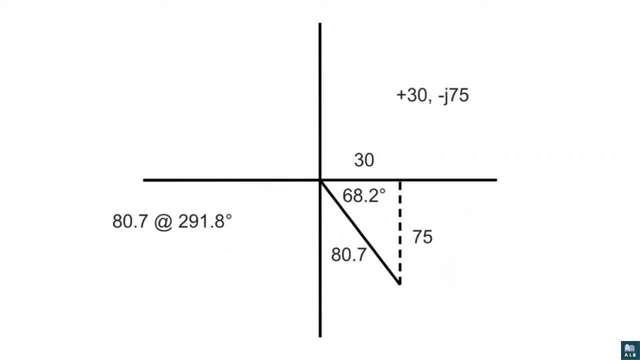 what we can also say when we're dealing with the fourth quadrant is: we can work our way backwards. Now I won't go too much into the why we can do this. you can do this with every quadrant, but we'll do this with the fourth quadrant because it's somewhere between zero. 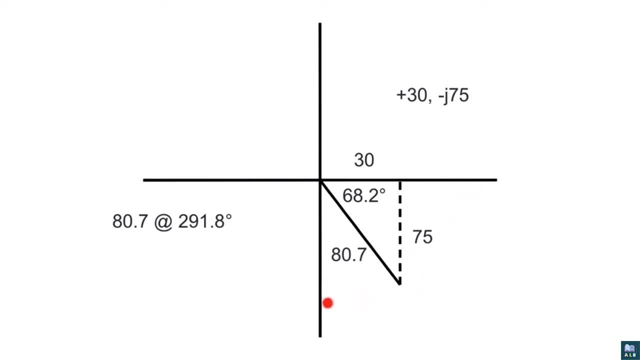 and 90 backwards. So it'd be zero and negative 90. This way we can look at it and say, okay, we got 80.7.. Add an angle of negative 68.2 degrees. it's the same thing as long as you work backwards. 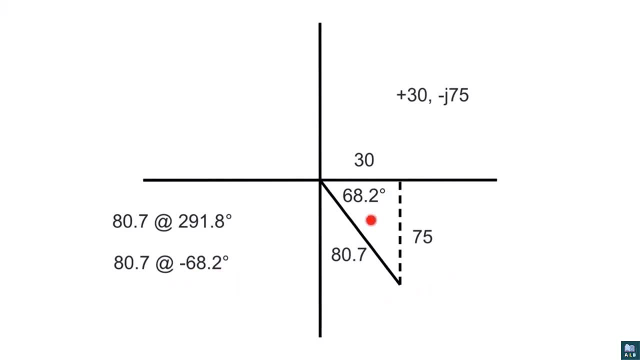 and we generally only do this in the fourth quadrant. So you can work out what this degree, this angle, is and throw a negative in front of it using this resultant, And you can work out what that is. Now it's very important that we understand how to do these conversions. 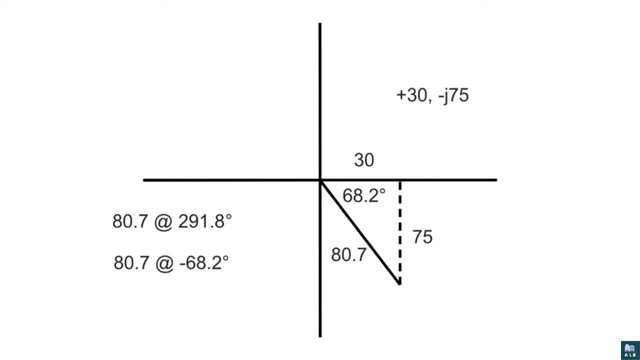 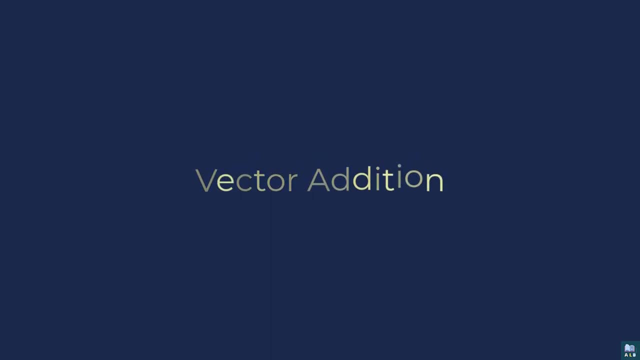 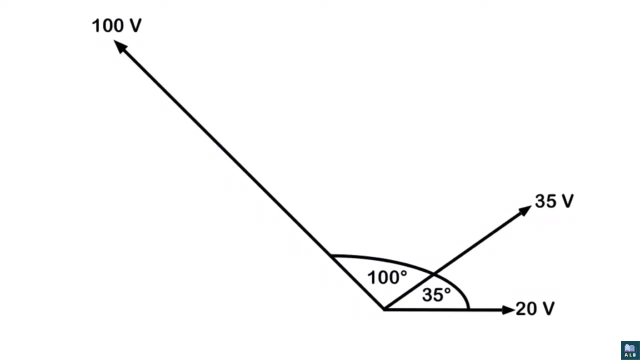 Because in our next video we're going to start talking about how to add vectors. See you there, Subtitles by the Amaraorg community at these. we're going to use this 20 volts as a reference. So I'm going to say that this guy here. 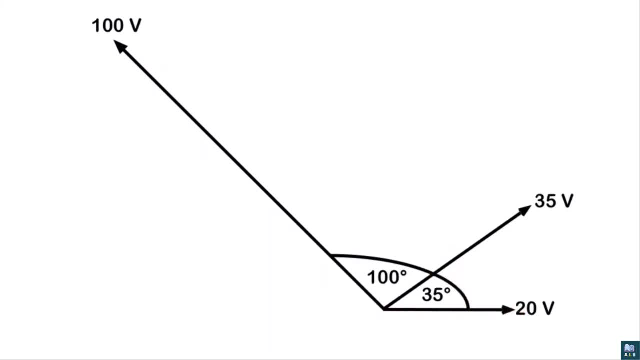 is 20 volts at zero degrees. I've got 35 degree angle in here, So this will be 35 volts at 35 degrees, And then beyond that I have a hundred degrees, So I'm going to add that a hundred to. 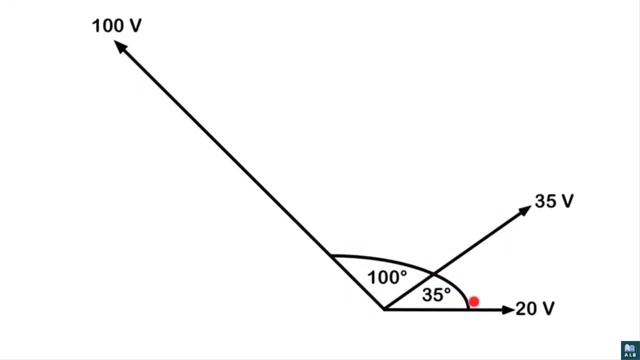 the 35. So I'm going to say I've got a hundred volts at 135 degrees. Now the first thing we want to do when adding any vectors is we want to put up our X- Y chart. So I've got myself an X. 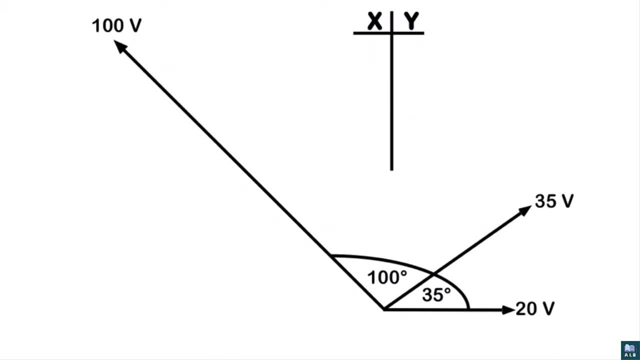 Y chart up here because it gives me a reference. Then I start figuring out what my rectangular version of these polar forms are. So I'm going to take 20.. I've got 20. at zero It is all X. So I've 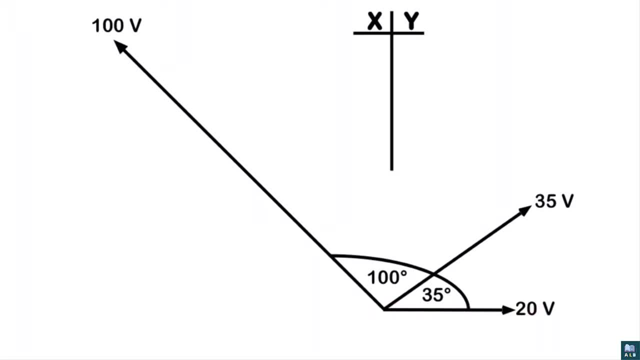 got 20 X and zero for the Y, So we're going to get that plugged in here. Now for this guy. here I've got 35 volts at 35 degrees. So what I'm going to do with that is I'm going to take the cos of 35. 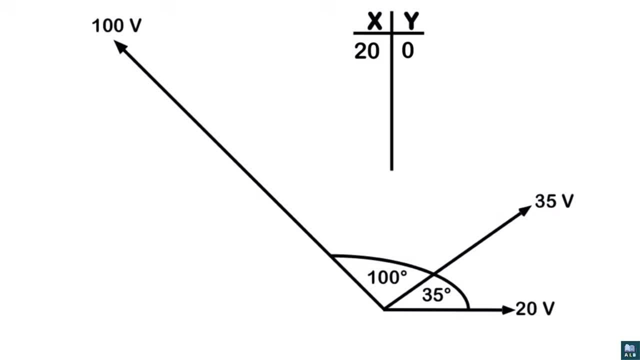 degrees times 35 volts and I get my X. and I'm going to take the sine of 35 degrees and multiply that by 35 volts to get my Y And that gives me 28.6 on my X and J 20.1 on my Y. And my last one here is just going to take the cos of 135 degrees. 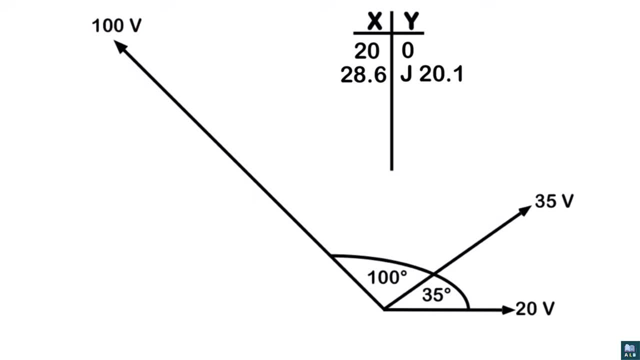 times 100 volts will give me my X, and the sine of 135 degrees times 100 volts gives me my Y. So plugging that into the calculator, I get my X being negative 70.7.. And I get my Y being 70.7 as. 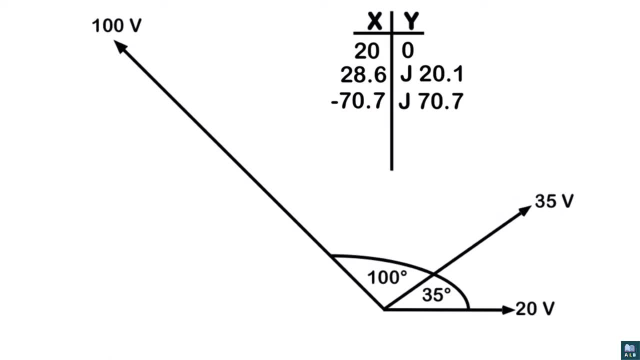 well, except it's negative 70.7 here, because we can see that if I drew this into a quadrant system, this vector here is in my second quadrant, So it'd be a negative X and a positive Y. Now I go ahead and I add up all my X's and I add up all my Y's and I get my rectangular version. 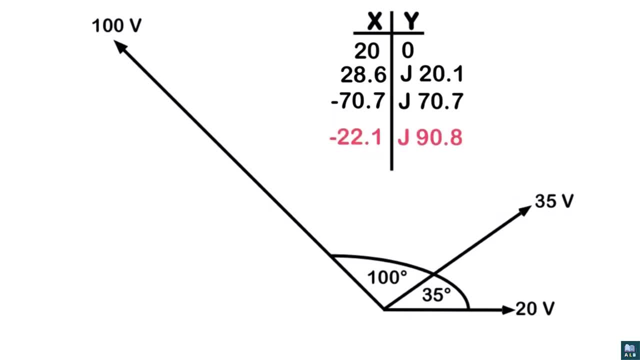 of the addition of these vectors. So I get negative 70.7.. And I get my Y being negative 70.7.. And I get my Y being negative 70.7.. Negative 22.1 for my X and J 90.8 for my Y. Now, I've got a bunch of numbers here, So what I'm?